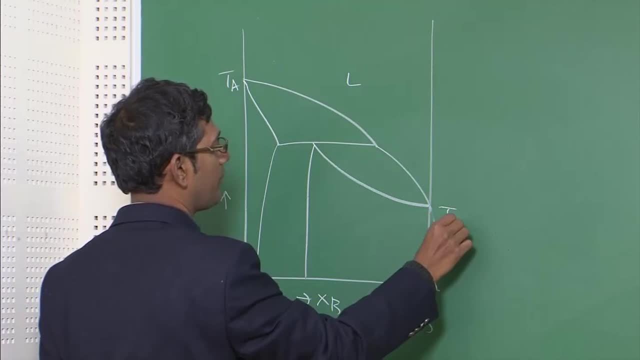 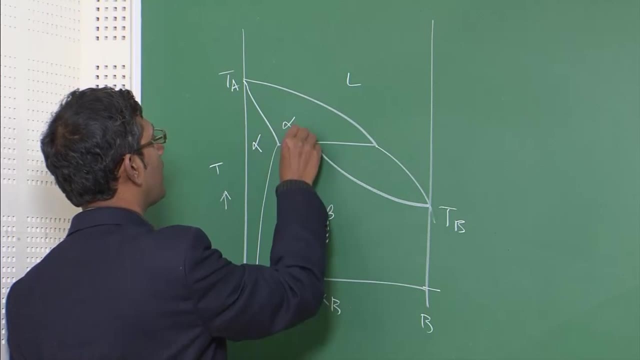 is the liquid. Let me first draw the melting temperatures of A and B. This is alpha beta and this is alpha plus liquid. This is beta liquid plus beta, correct? So this has a peritectic reaction at the peri temperature Tp. But I told you that most of 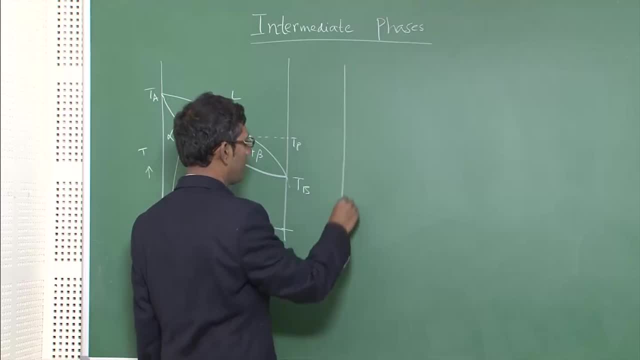 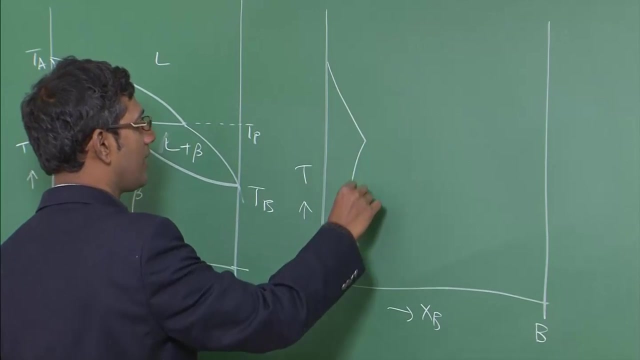 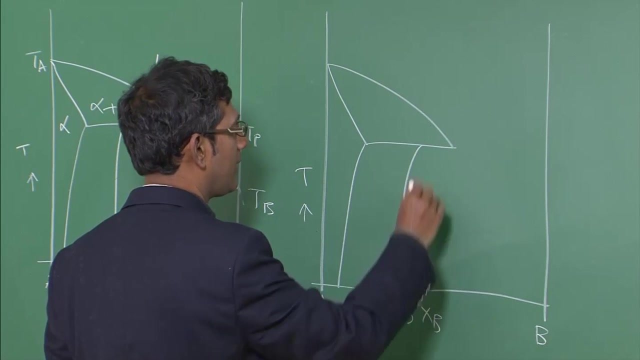 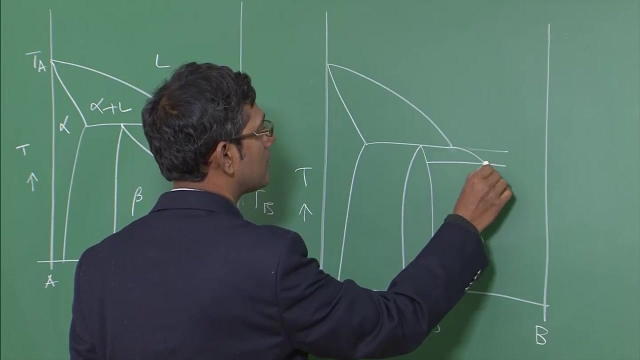 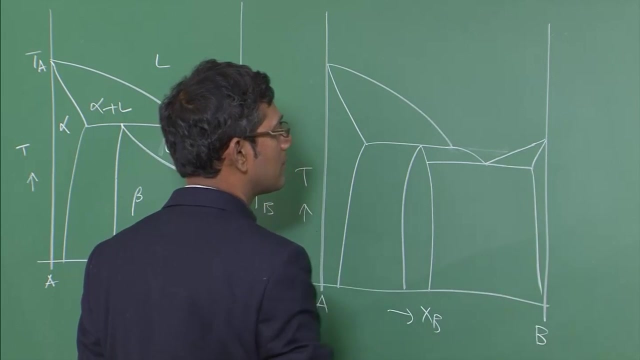 the peritectic reactions are followed by eutectic reaction. So, and this is where the intermediate phases forms. So let me again draw the modification of this diagram, or little different from this. So first is again remain same, Then you have this and there is a separate. So this: 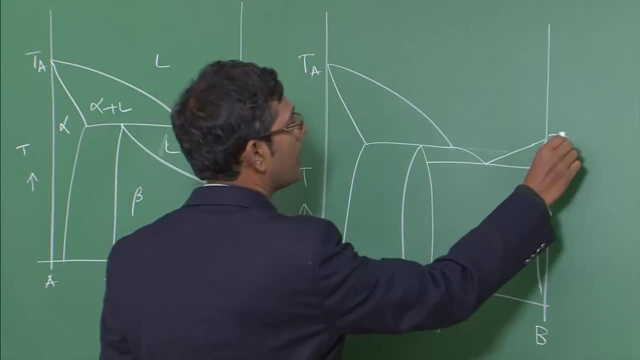 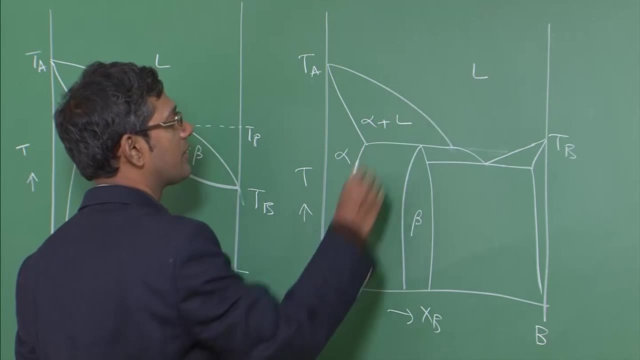 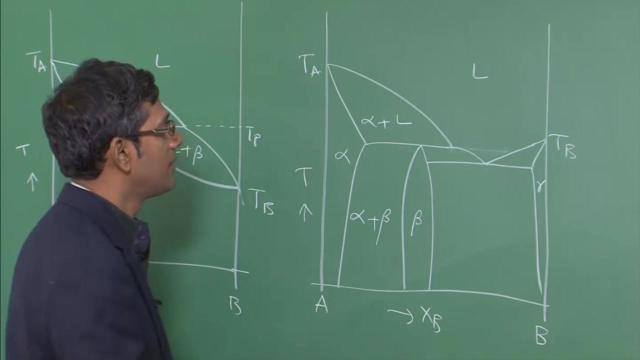 is what I am trying to say. So the melting temperature of A, melting temperature of B- liquid alpha, this is the beta. Therefore, this is liquid plus alpha, alpha plus beta, and there is a new phase, gamma correct. So this phase forms by eutectic reaction from. 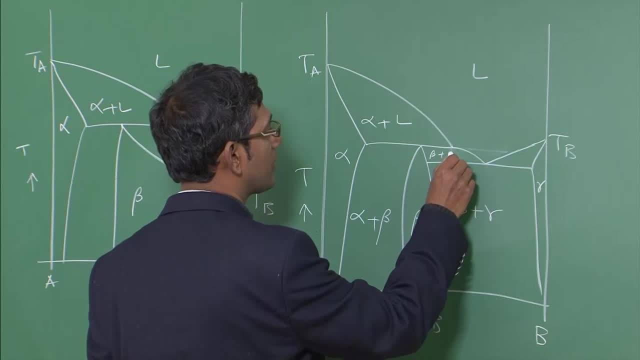 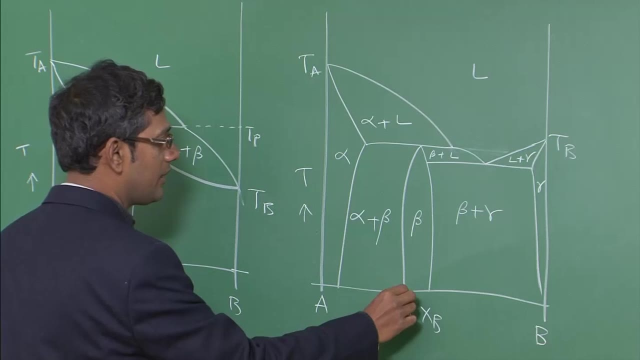 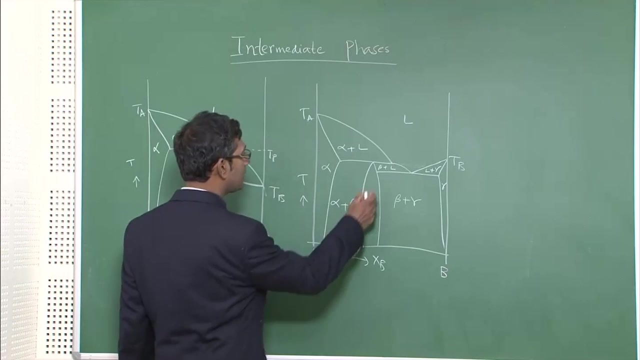 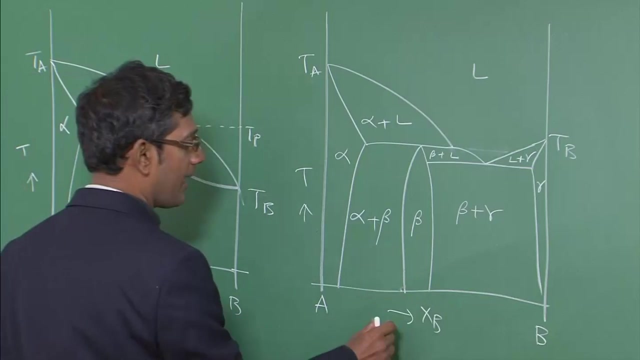 the liquid. So therefore this will be beta plus liquid. This is liquid plus gamma. Now I am talking about this phase which is formed here. beta, Which is distinctly different from this. You can see here beta is composition, is only sitting at the center of the compositional axis XB almost, and it has a small span. It 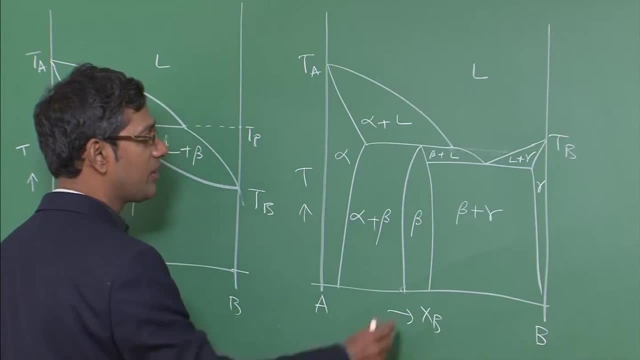 is not exactly a line. It has a small span of composition in which it is stable, and this normally has a different crystal structure. So such a kind of phases are called intermediate phase. The reason it is called intermediate phase is because of this. 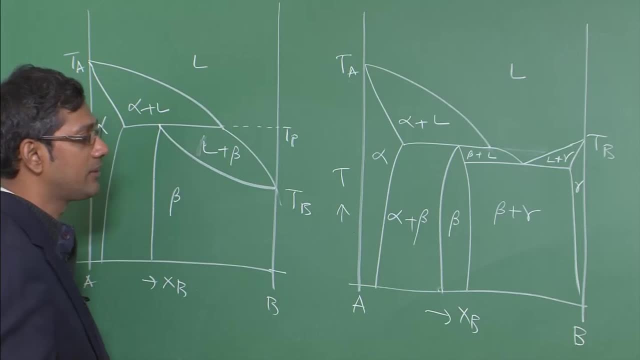 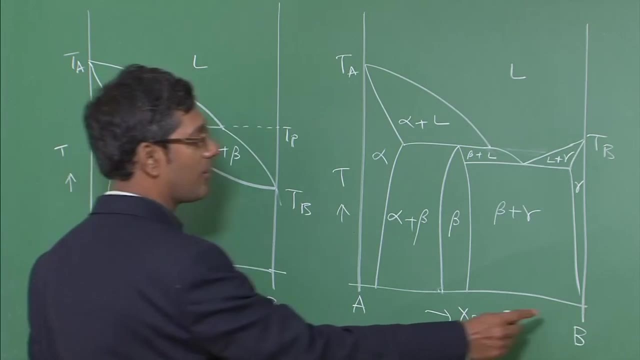 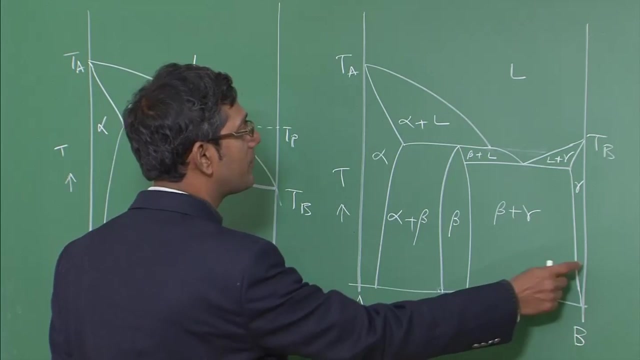 We know that there are two solid solutions at the end or at the terminal positions of A and B respectively. One is alpha, which is A-rich solid solution, other one is gamma, which is a B-rich solid solution. Now this phase comes in between of this composition. 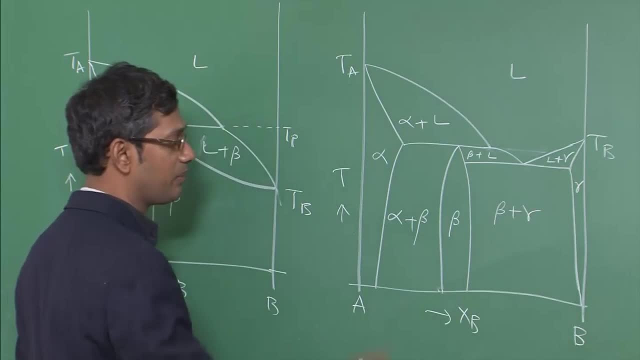 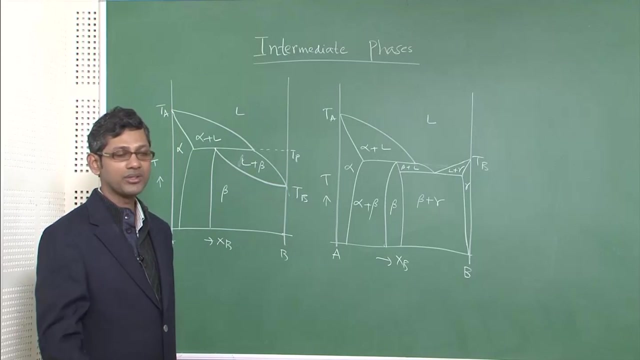 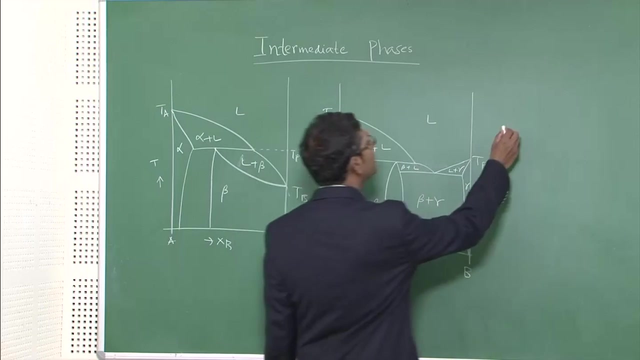 or intermediate compositions of these two solid solutions. The beta comes intermediate compositions of alpha and gamma and that is why it is called intermediate phase And because it is does not have a fixed stoichiometric composition like sodium chloride, potassium chloride or any other phases, it is called intermediate phase. So intermediate phase. 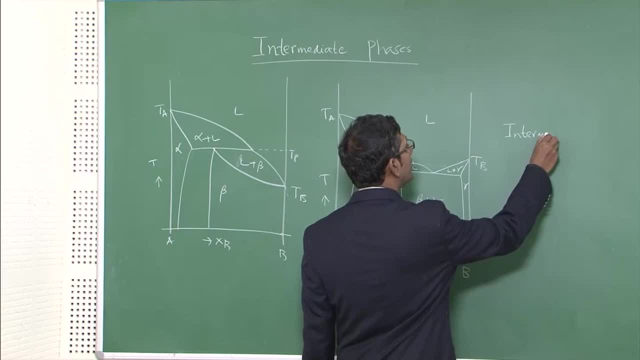 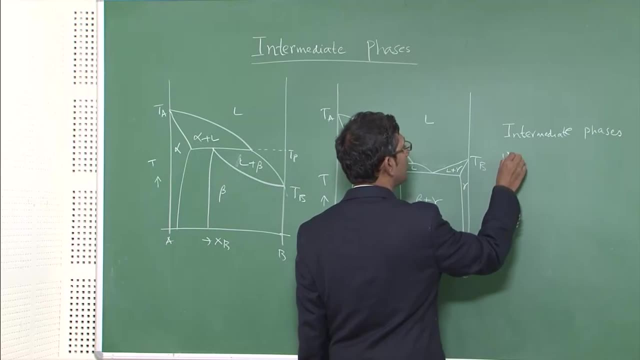 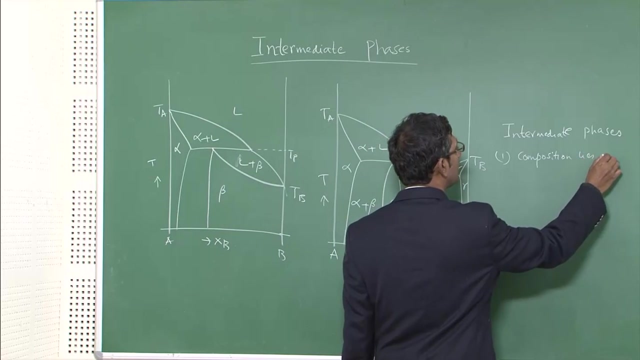 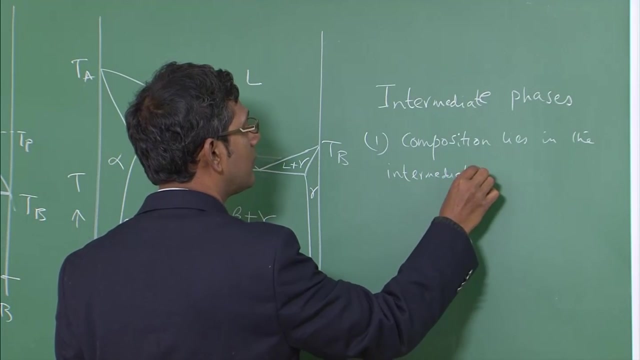 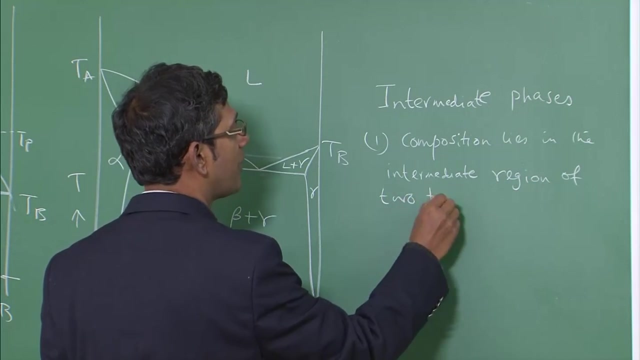 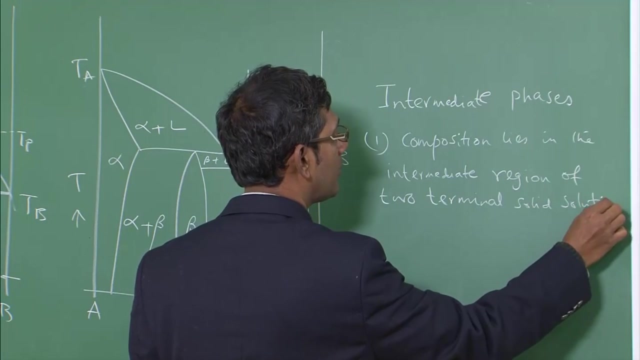 means its compositions lies intermediate of two solid solutions at the ends. So first is the composition Composition lies In the intermediate region of two terminal solid solutions. That is the first thing you will see for this kind of phases And this is very common, As I will show you in a quick. 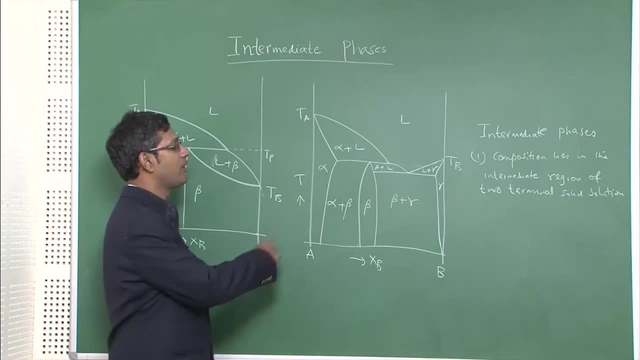 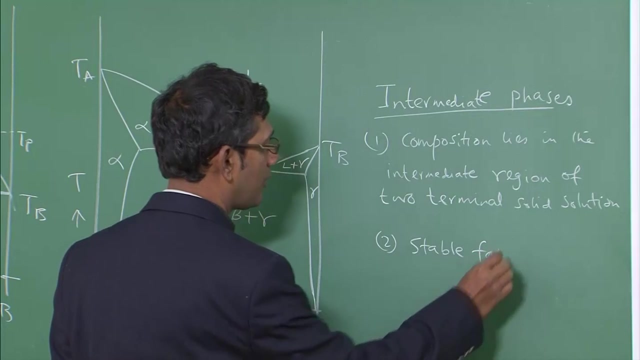 slide After some time how these phases will appear in the phase diagram. So this is the first condition to be satisfied for the intermediate phase. Second condition to be satisfied is that this phase is stable for a small compositional range. What I mean to say is: this is not a 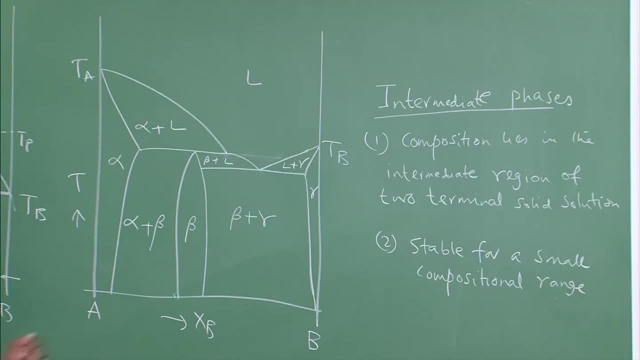 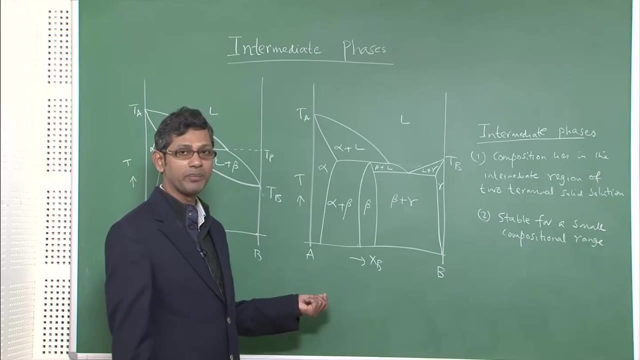 compound. If it is a compound, then it will have a fixed composition, But it is not. It has a range of composition in which it is stable. It may be 2%, it may be 1%, it may be 3%. It does. 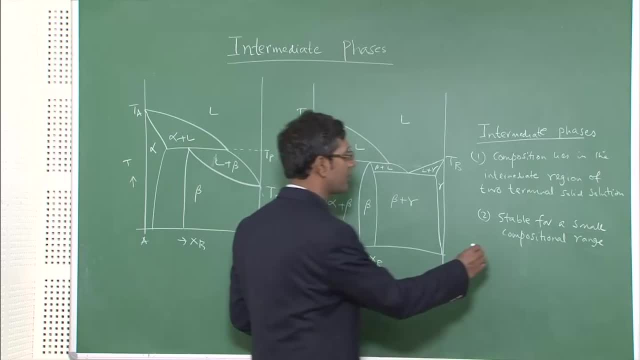 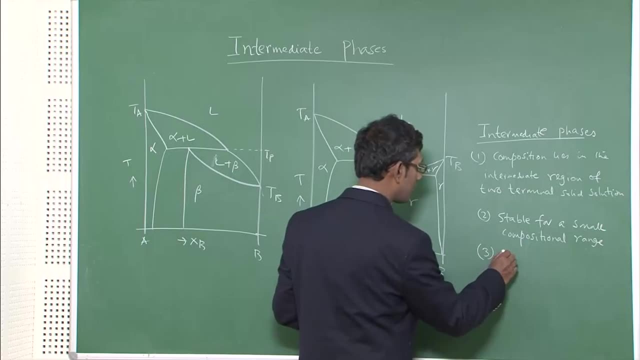 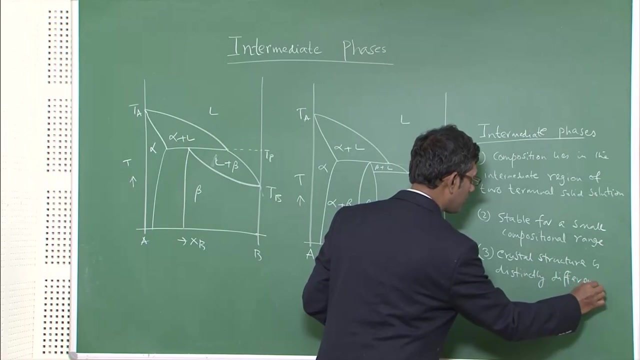 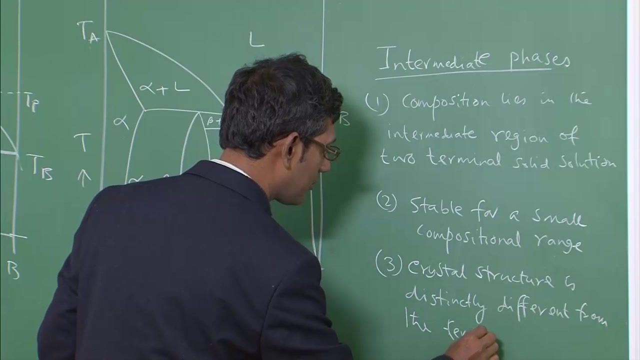 not matter, But it has. Third important criterion to be satisfied by these kind of phases is that the crystal structure of this crystal structure of this phase is distinctly different from the terminal solid solution And therefore they are distinctly different phases. They are not the same as either of. 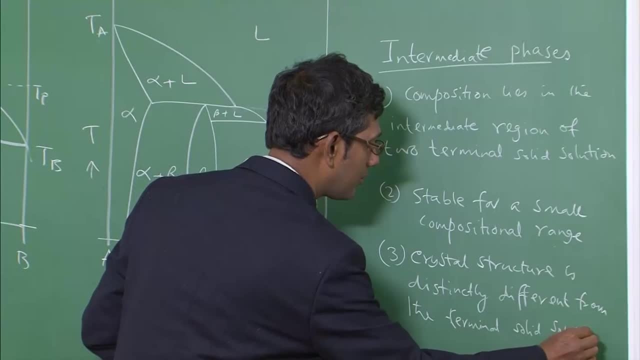 these two terminal solutions, And they are distinctly different: intro, top and quasi extension. zuz wish급ği, two tens rebuilt, Only one being upright For jumping the 옛날 level paper. Finally, another thing to make sure is this: Because the temperature here appreciate a very, very important point in this particular problem is: currently we have a fine pour into this specific comment- It is possible to turn a water mark with only by ethnic increasing at 1% per minute, Since thisaps in time comes to the concentration reaching form of lowest in matter per. 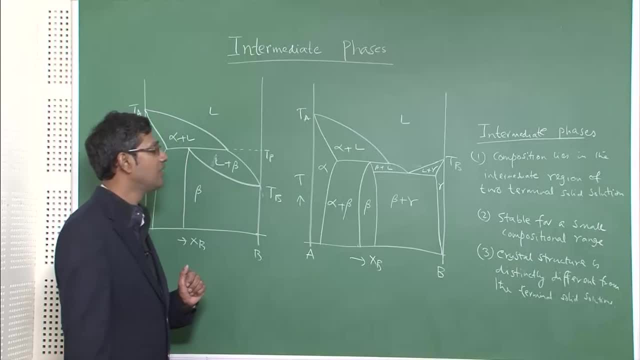 sample number. Some of the other two donner applications are common in bestimm regions k. Now we shall look at some more�� times. So let me look for this particular point in this particular operators, and they are distinctly different phases. So you have already got an idea that such a kind of phases exist in the peritective. 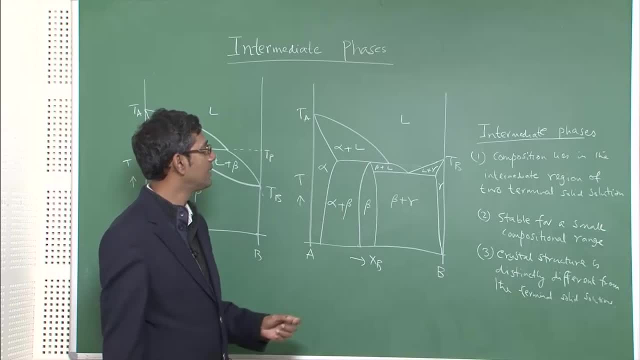 phase diagram. As you see here, it forms by peritective reaction. In fact, this phase diagram I have already shown you at the beginning, that is for the iron carbon phase, iron germanium phase diagram, in which there is a phase called epsilon which forms out of the peritective reaction between alpha and liquid. 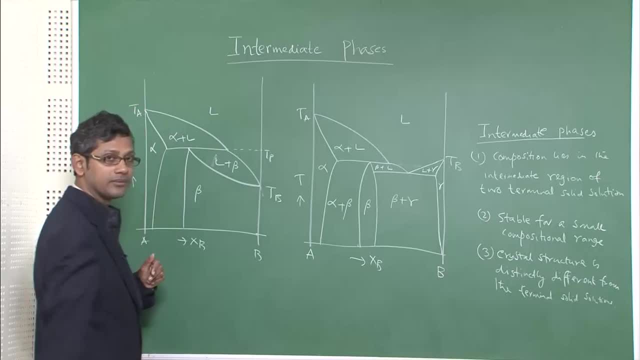 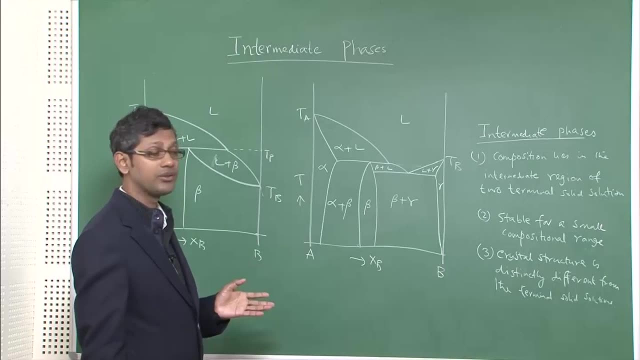 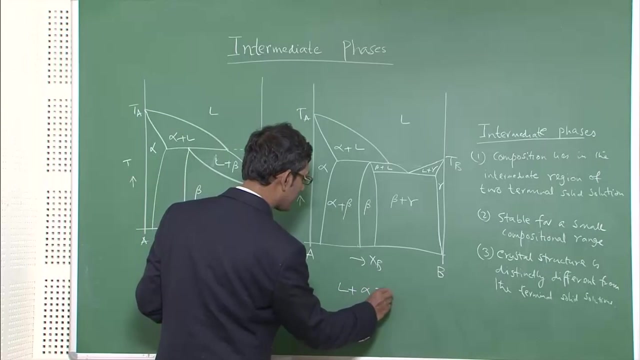 So in this case beta is a solid solution which has extend from this to this. but in this case beta is an intermediate phase. it is not a solid solution. that is the difference you must make out from this diagram. Here beta forms by this reaction. here also, beta forms by this reaction, same reaction. 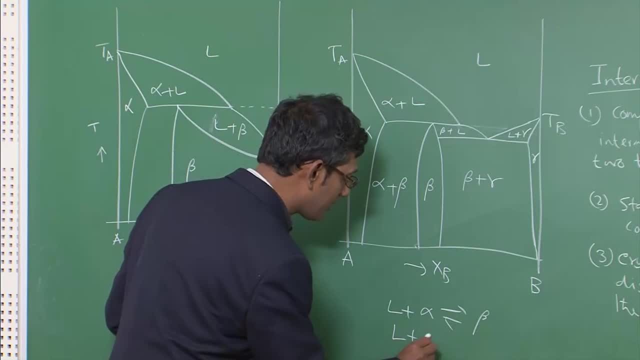 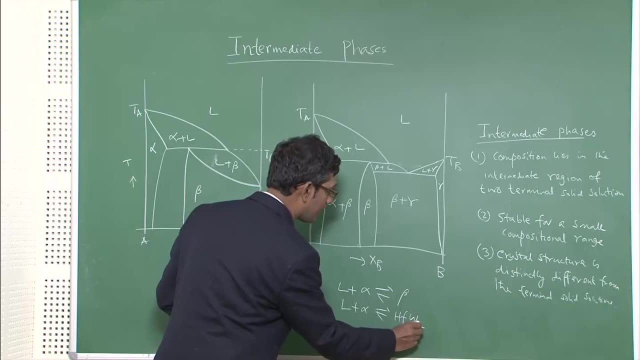 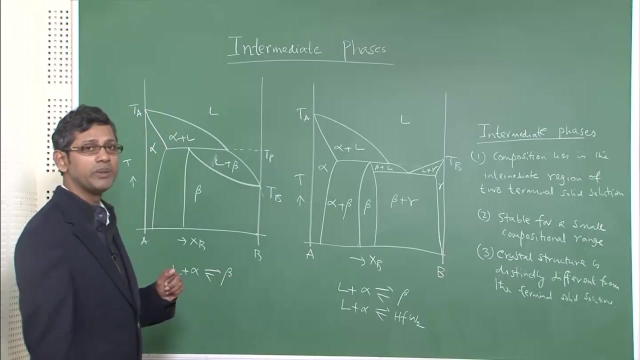 but things are different. One example of this is in hopium Tungsten phase diagram there is a phase called HFW2 forms as a reaction, peritective reaction. So there are many host of phases. Now, with this brief introduction I have given you, let me just show you few phase diagram. 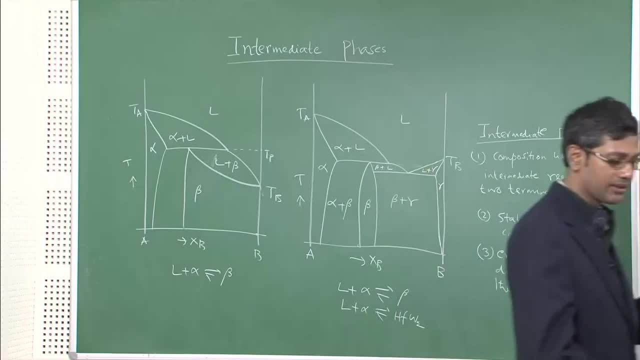 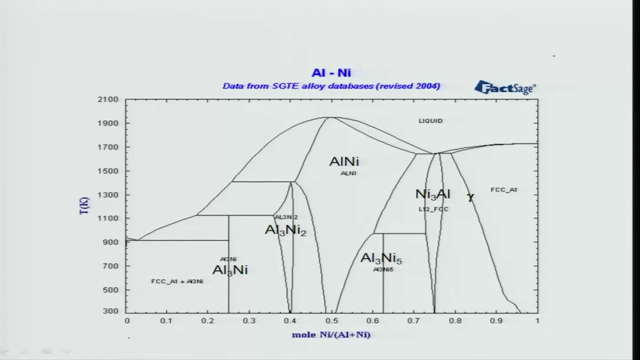 why such a kind of phases exist, and then we will discuss further. So let me just take you through the phase diagrams. so which will come alone? and here it is. This is the first phase diagram I am showing you aluminum, nickel. You can see here I have written many phases like Al3A9, Al3A2, Al3A5 and Ni3Al, all of 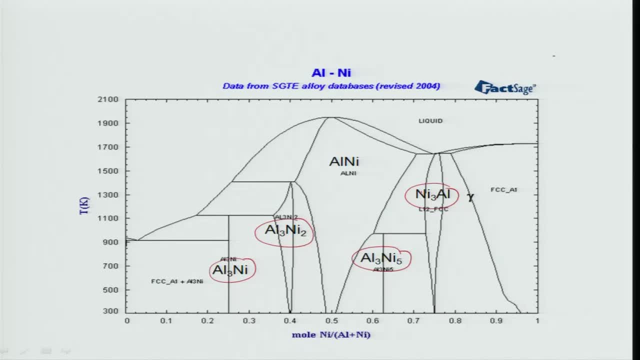 these phases form by peritective reaction. all okay, But you see, Al3A9 is a line, as a line like this is a line compound. Al3A5 also is a line compound, Okay, But on the other hand, Al3Ni2 and Ni3Al has a stoichiometric, has a compositional range. 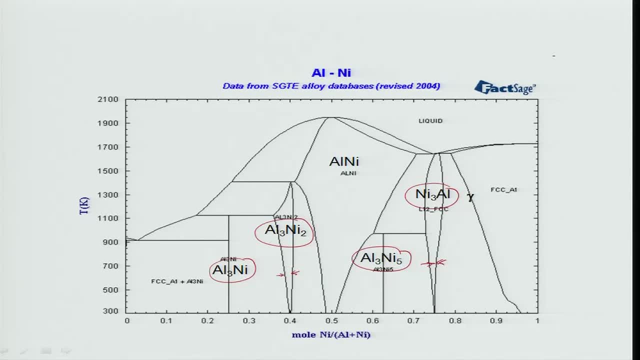 in which it is stable. It is not only a line, but there is a domain range of composition is stable, okay, So therefore these phases are called intermediate phases because their composition lies in between the solutions of nickel and aluminum. There is another phase called AlNi, here with composition AlNi, which has a large compositional 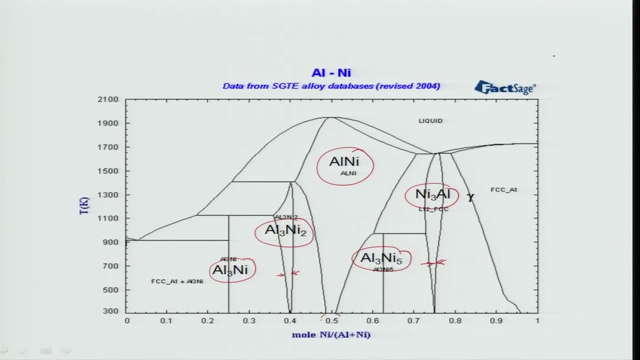 stability range. It is not formed by peritective reaction, by a different one is called congruent solidification or congruent melting. melted compounds. it directly forms from the liquid, But all of them forms by peritective reaction. Here you see, there is a peritective reaction, there is a peritective reaction, there is. 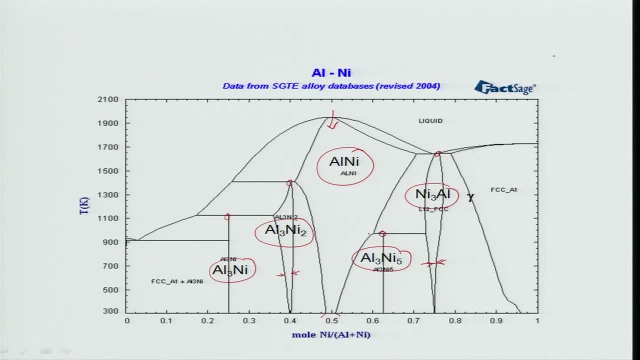 a peritective reaction and there is a peritective reaction there. So this is a classic phase diagram, but you know all of these are useful material. Most important one is Ni3Al, which is used in the real applications. All these phase diagrams are useful. 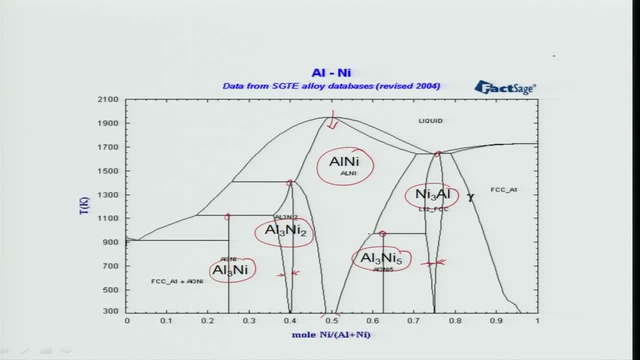 All these phase diagrams are useful. All these phase diagrams are useful. All the turbine blades which is used in the steam generators or even the jet engines, they are made of this alloy. Ni3Al precipitates- Gamma gamma 1 precipitates- you might have heard about it. 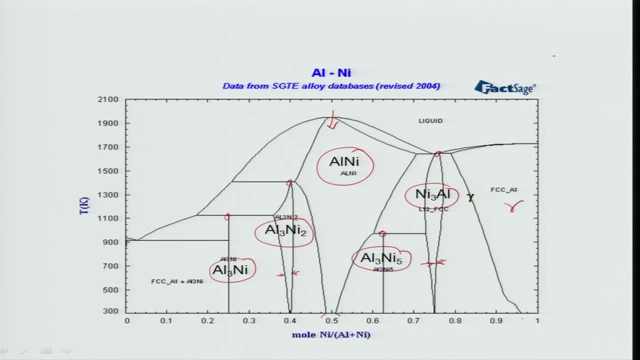 So gamma, is this FCC solution of nickel? okay, and gamma prime is this Ni3Al precipitate? So this is the first example. remember these phase diagrams are all available online from the SGT website or FACTSTAGE website, So you do not need to look into any book. they are available free. 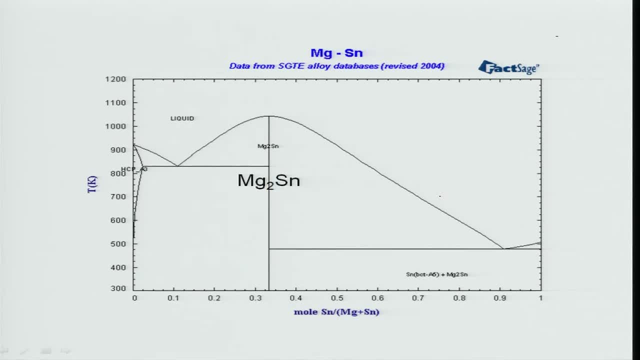 Now let us move on. there is another compound here I am showing you for MgTin system phase diagrams. You see, here there are two eutectic reactions in MgTin system- eutectic I have already discussed- And in between there is a compound, Mg2Sn, as a line. okay, it is a fixed stoichiometric. 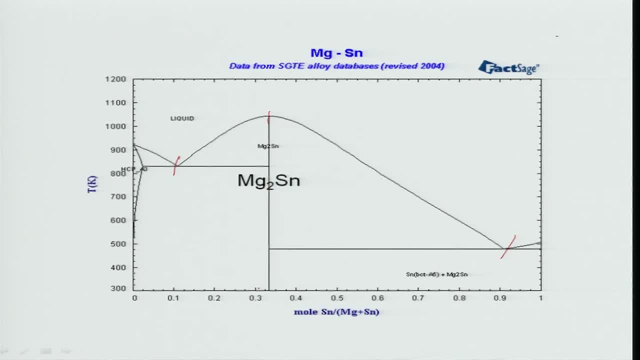 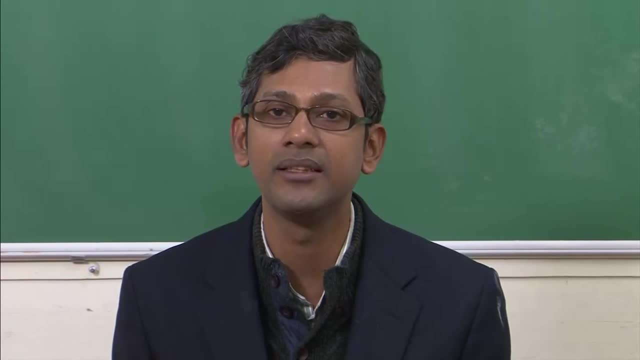 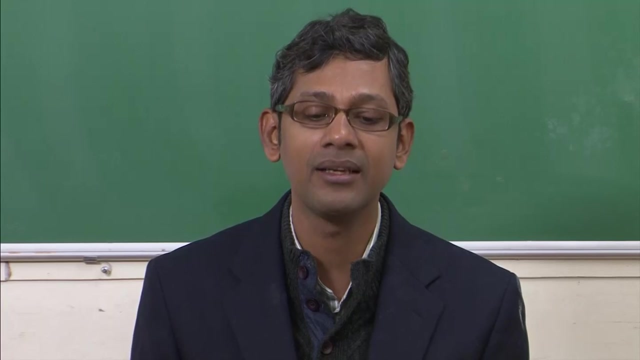 compositions. Okay, There are many intermediate phases where this fixed stoichiometric compositions are maintained. but, as I told you in the very beginning, that is not necessarily the condition to be satisfied by the intermediate phases. there can have compositional domain range, But examples do exist where the compositions is fixed and then there is a line in the phase. 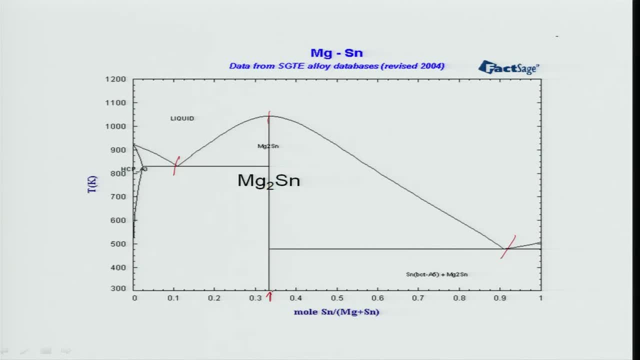 diagram. So whenever you see a line that means there is a fixed stoichiometric compositions for the phase existing. So here Mg2Sn is forms at the fixed compositions. It has eutectic reaction between the solutions of pure Mg. pure Mg is alpha Mg- okay, plus Mg2Sn. 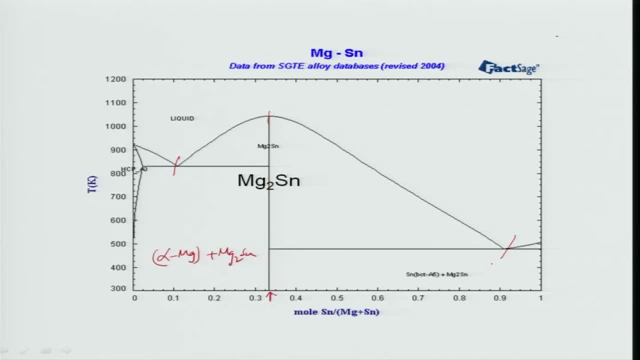 On the other hand- here you can see- it is Mg2Sn plus the tin phase. So Mg2Sn plus beta tin is eutectic. Very simple phase diagrams, Okay. Only difference is that there is an intermediate phase at the center, almost 33% of tin. 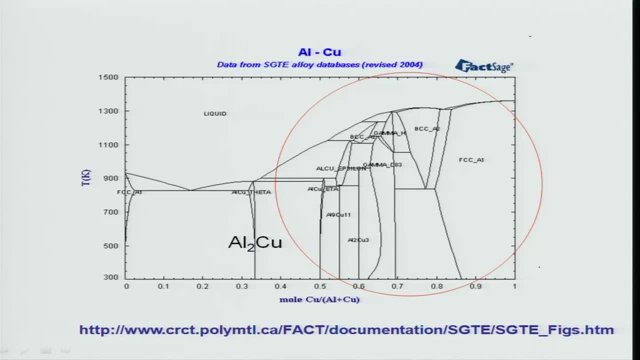 Now for aluminium copper. there are many, many, many, many phases. I cannot discuss even that. So region I marked like magenta color circle. there are many, Let us not discuss The starting one is Al2Cu and it has high temperature. it has a slightly larger compositional. 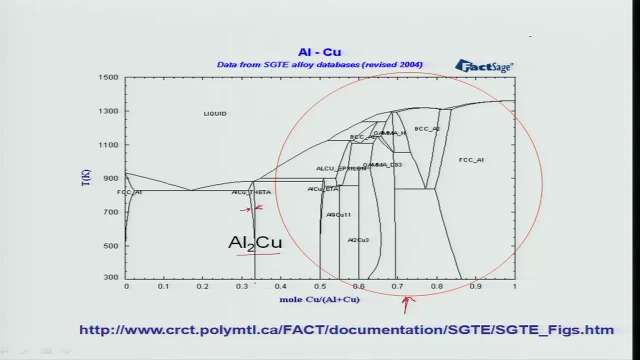 stability zone but lower temperature. it has a fixed compositions. Then you have Al9Cu. Okay, So Al9Cu11, Al2Cu3, there are many others phases which exist with a compositional range, and some of them AlCu, AlCuC or AlCu forms by eutectic reaction. even Al9Cu11, it forms. 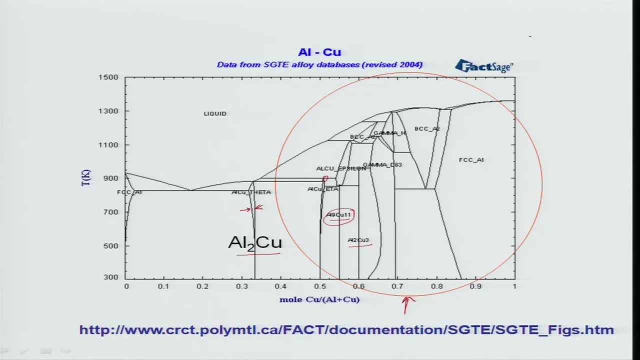 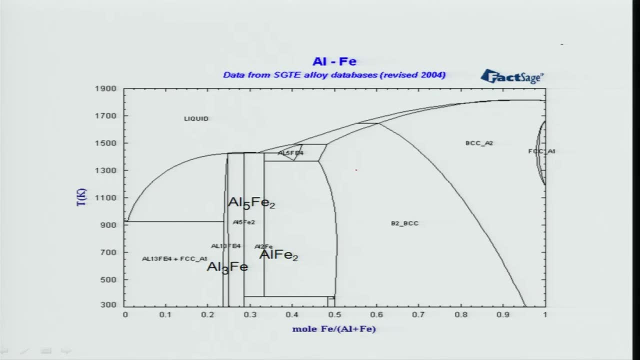 not by some other reactions, but on the other hand, Al2Cu3 is formed by eutectic reaction. So most of the intermediate phases forms by eutectic reactions. Now another important phase diagram where this intermediate composition, Okay, So this intermediate compounds exist in large or in several ones. exist in aluminium, iron. 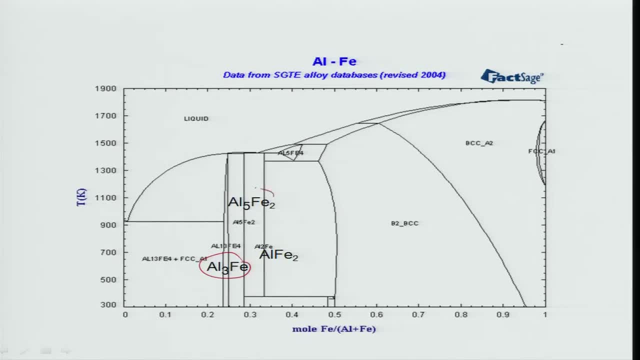 This is what I am showing you. You can see there is Al3Fe, Al5Fe2, AlFe2 present and there is another one, Al5Fe4, at the top, Correct? So all of these are actually intermediate phase. and this one, this one, also this one. 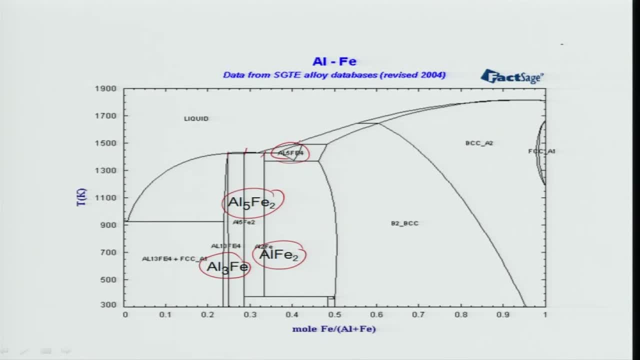 all of these three are even this one. All of them- Okay, All of these are actually here- are forming by eutectic reactions. So you have to simply look into their phase diagram, database or data to see what is the which phase it reacts with liquid and form this eutectic reactions. 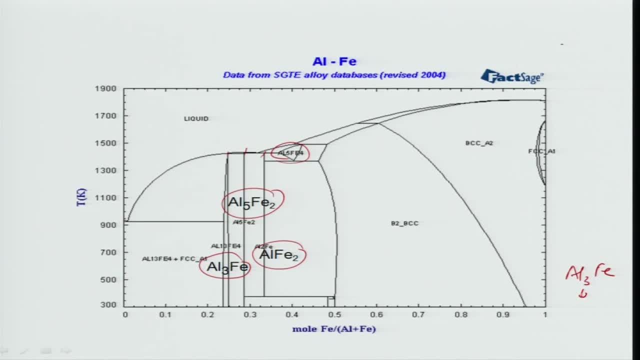 Sometime Al3Fe is written as Al13Fe4 because of compositional deviations. but you can see Al3Fe has a compositional range. On the other hand, other two has no compositional range in which it is stable, but it is stable only for a fixed composition. 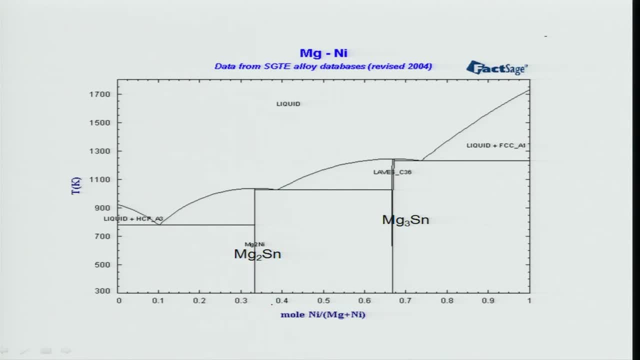 That is Al3Fe. Now let us look at. this is another very classic phase diagrams: MgA9. MgA9 has two intermediate phase: Mg2Sn, for a tin composition of 33%, and Mg3Sn- tin concentrations of about 66%- 66.66% of tin here, and these are called Lavish phases, which we will discuss. 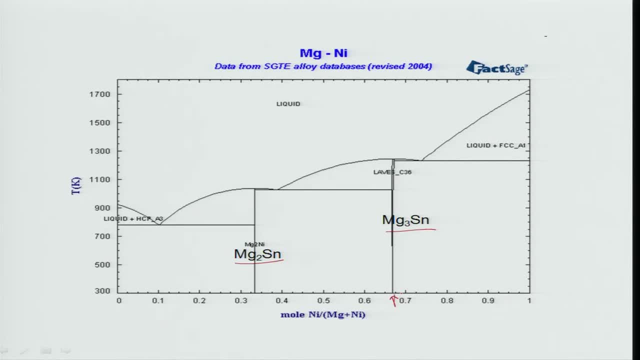 later. what is Lavish and who discovered How? There are some characteristics of that, but you know, both of these three phases has eutectic on the two ends, correct, But these also forms by a peyotric reaction. This also forms by a peyotric reaction. 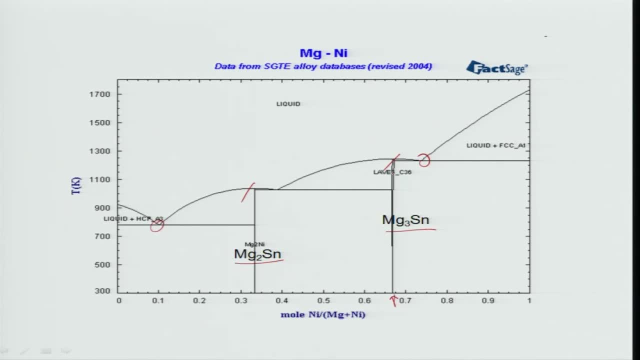 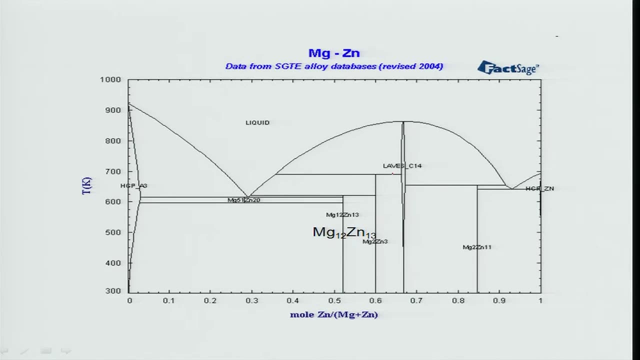 Now this does not form. This forms congruently from a directly from the liquid, but this forms a peyotric reaction. Mg2Sn, MgZn- again a complex phase diagram, but one can see there are several phases- Mg12Zn3,. 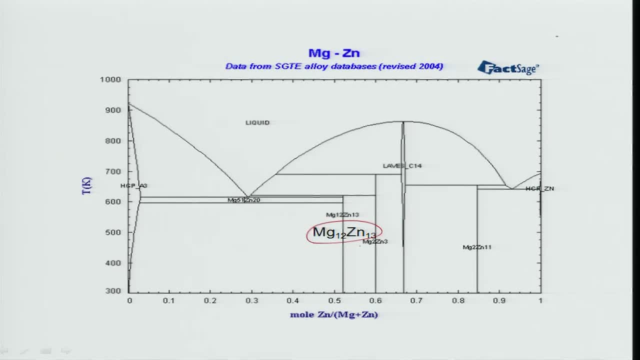 Mg2Zn3,, Mg2Zn11,. this definitely form a peyotric reaction. this definitely form a peyotric reaction. this one, also all of them, and there is another phase at the center which does not form a peyotric reaction but by congruent melting or congruent solidification is Lavish. 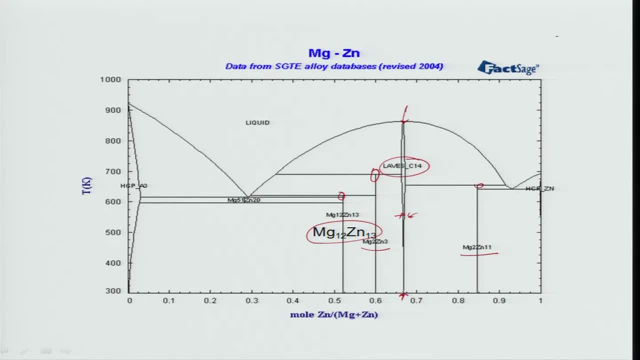 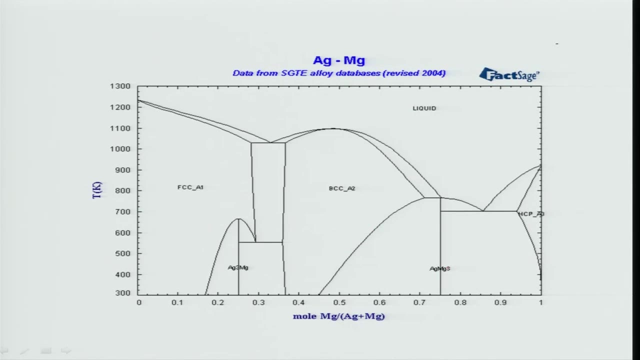 C14 phase, which has a composition about 66% zinc and rest of tin, So it will be Mg3., Mg3,, Mg3, what? Mg3, Mg3Zn. this composition. it will have Lavish phase, So you can. then there are others, like silver magnesium. most of them are actually with 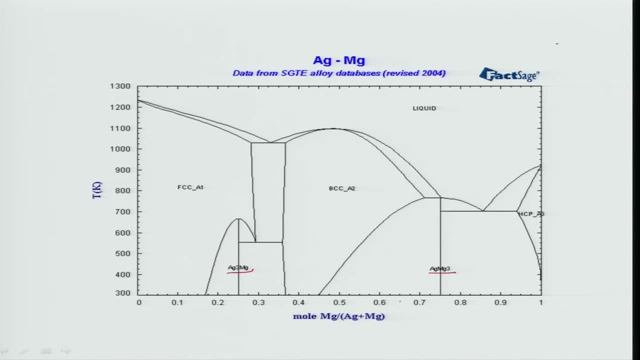 magnesium, Ag3Mg, AgMg3, there are two and AgMg at the center, But these two, Ag3Mg and AgMg3, they are, you know, almost like a line, But AgMg has a large composition domain. 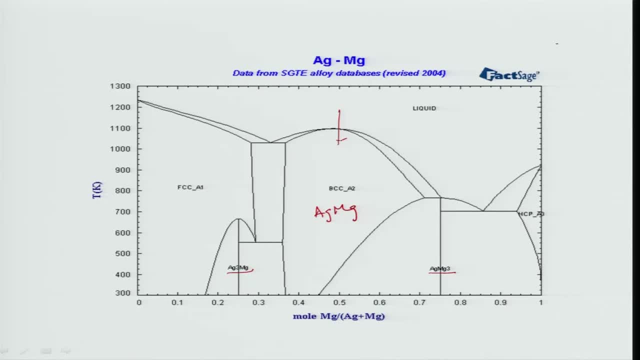 But AgMg does not form by peyotric reaction, it form by some other thing, like incongruent solidification, which we will discuss later. Silver copper, I have shown you Now. so therefore, all these phase diagrams I showed you, I will again showing you one. 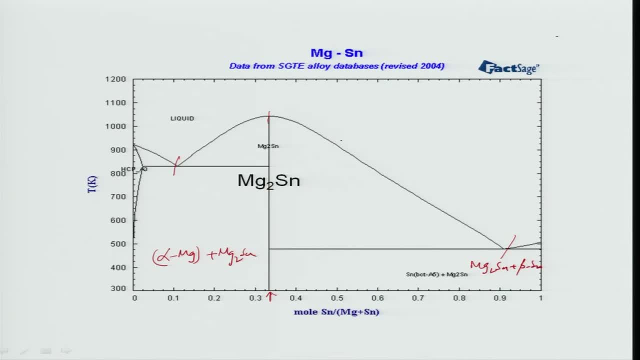 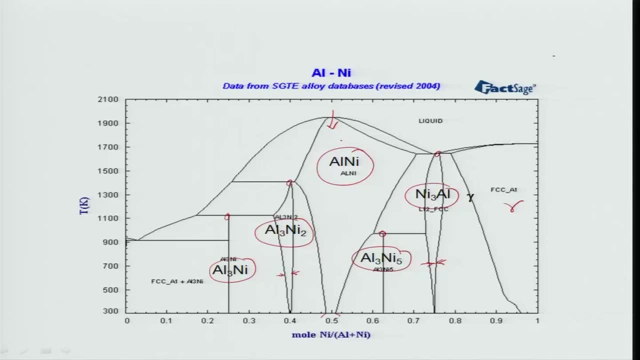 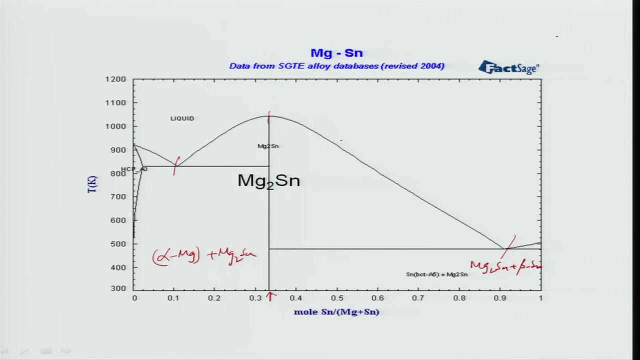 more time just flashing you to make you believe that these are actually real phase diagram, and these phases exist in the real phase diagram database. So thus it is important for us to understand. So now, with giving these examples of intermediate phases, let me just tell you that we can classify: 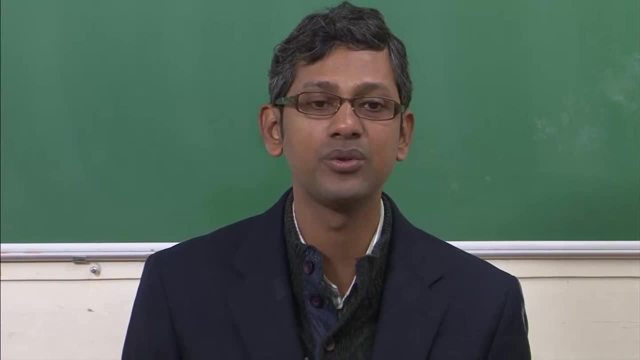 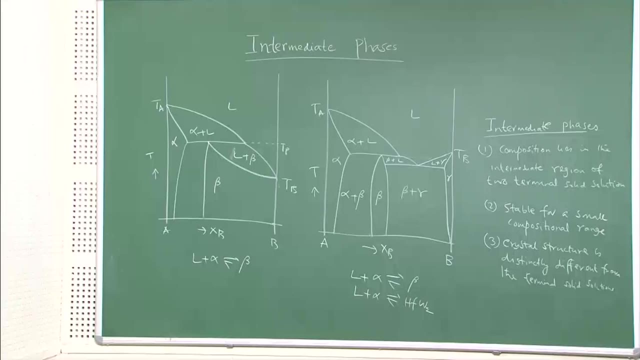 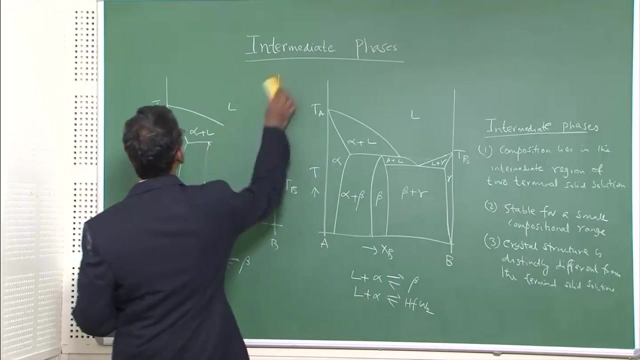 them because you are flooded with many phases and compositions. we can classify them as three types And that is what I am going to write you on the board and this is very important lesson you should remember. you should not forget. This is very important because these are the data not available in many books which I am 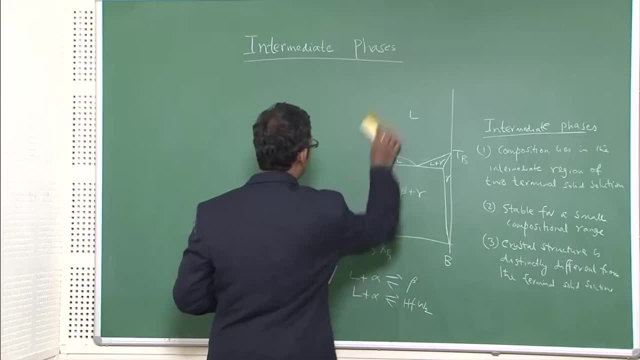 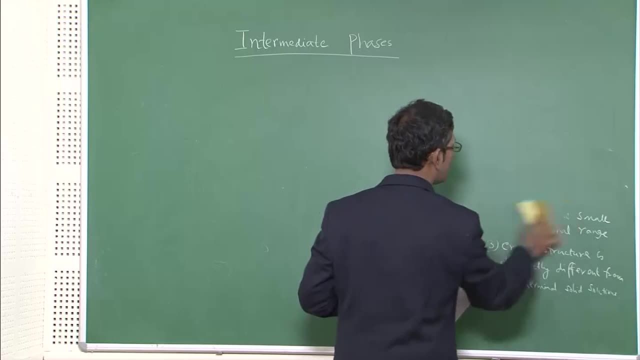 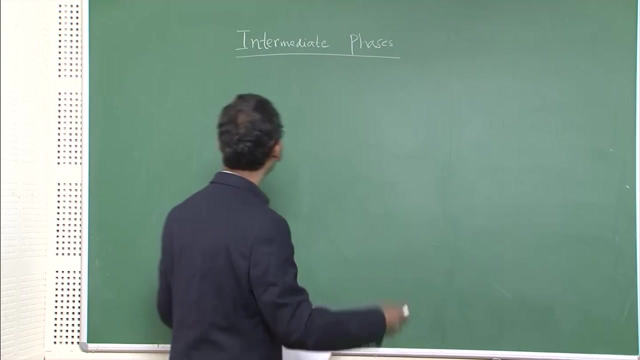 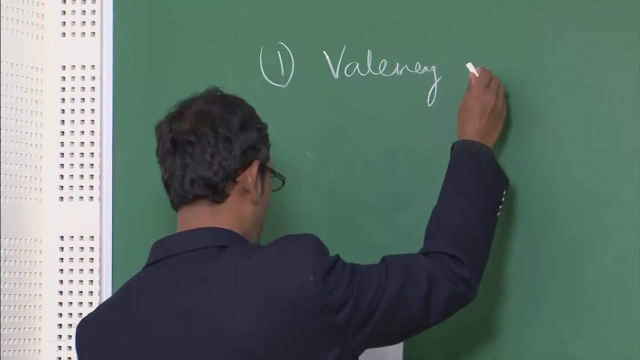 going to give it from this A particular sheet which I have taken down from the text book. So there are three types of intermediate phases. classically, The first one is known as valency type. First one is known as valency type or valency compound. they are called because they follow. 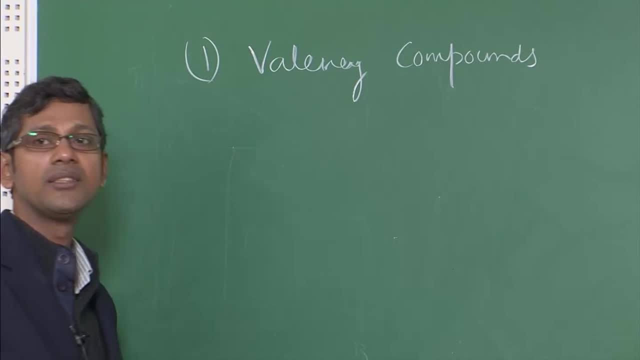 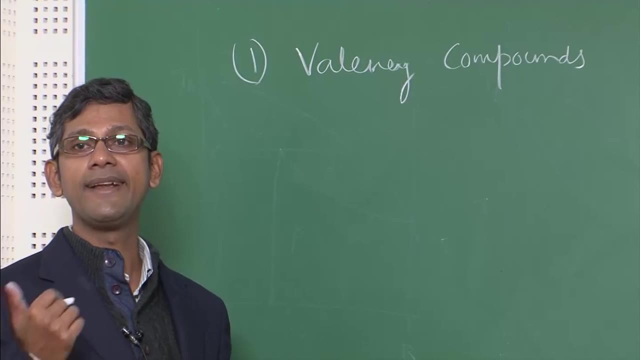 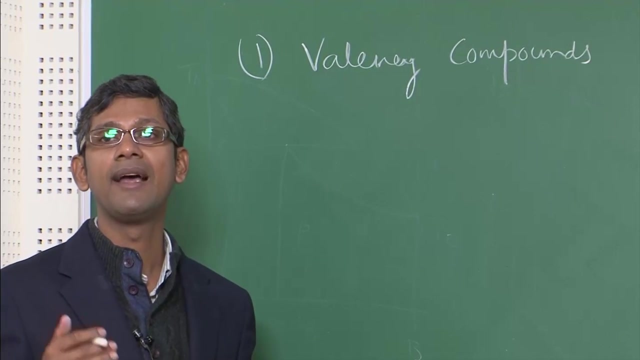 typical valency rule. What is that? If you consider sodium and chloride? sodium loses one electron and becomes octet at the outer cell and chlorine takes that one electron, become octet in the outer cell. That is how sodium become plus ion, positive ion, and chlorine becomes negative charged. 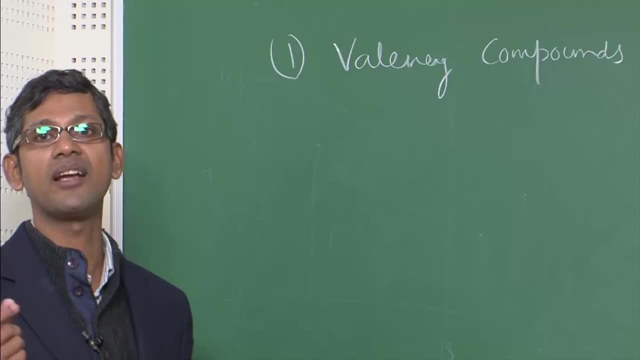 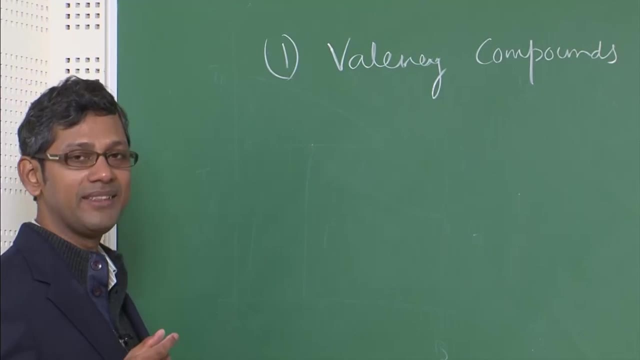 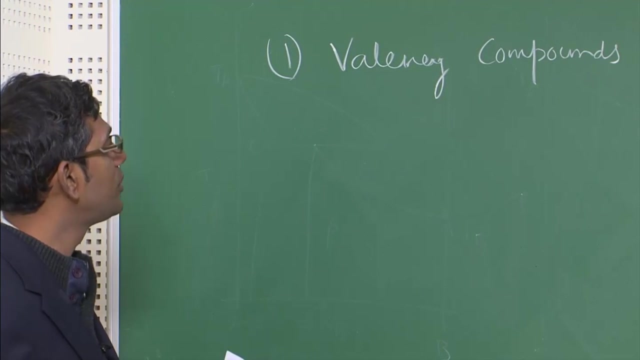 ion, and then there is a- you know- natural attraction and it forms a compound. So that is actually called a valence compound, because valency is meant, or electron transfer takes place at the valency band. So there are many such compounds which obey this rule and they can be of these two compositions. 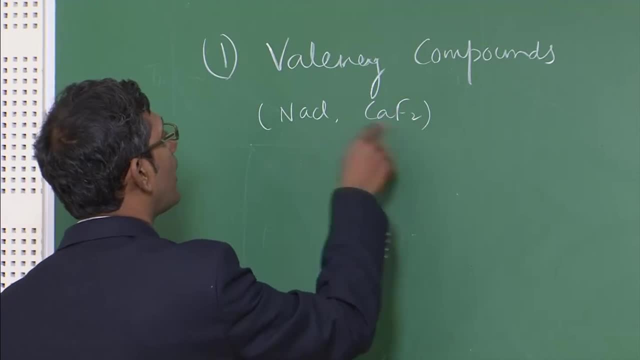 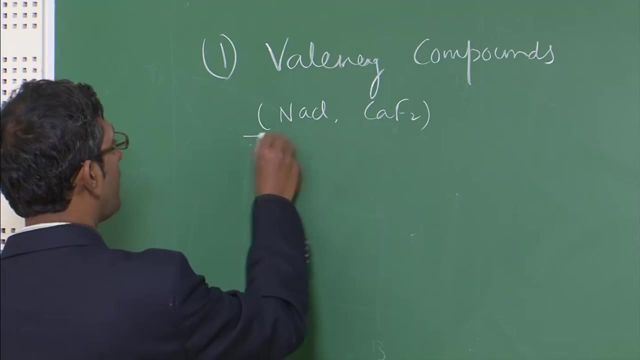 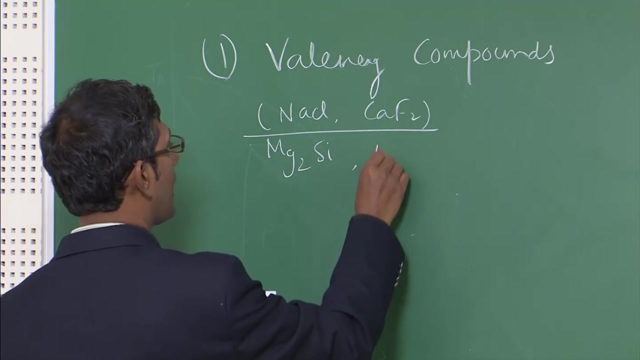 NaCl or Cf2.. Sodium chloride or calcium fluoride compositions. Both are ionic compounds, both are actually valency compounds. I will give examples in intermetallic phases. these are Mg2Si, Mag 2, Mg2Sn. I have shown you. 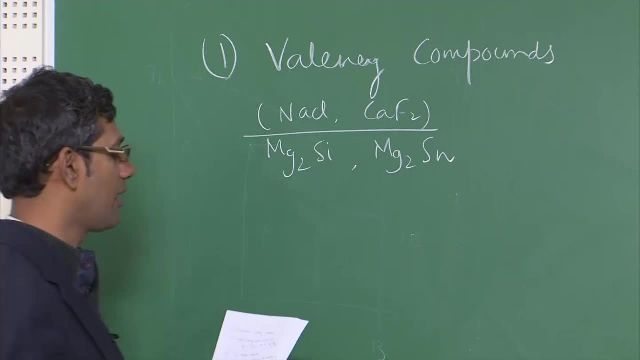 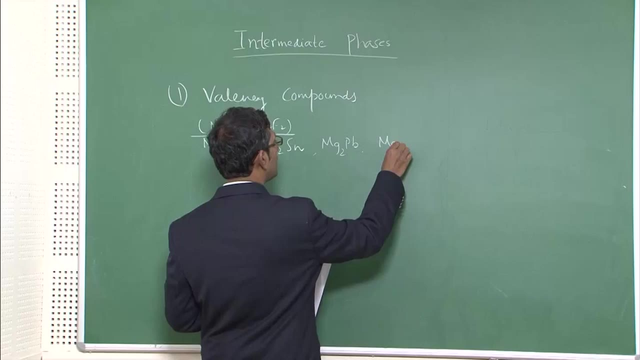 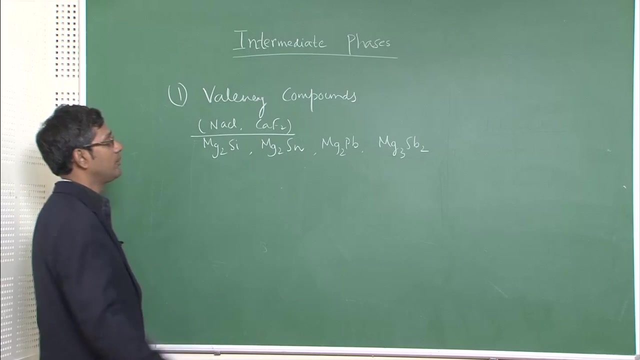 A valence compound which exists in magnesium think diagram, and Mg2Pb, another one. and last one is Mg3Sb2- magnesium antimonides. These are very important. you know, antimonides are actually thermoelectric materials. they are useful. The first type of compounds: they are called valency. second one is known as size factor. compound. Why they are called size factor compound? because they are stabilized by size factors, or difference of sizes of the atoms, different sizes of atoms. just like we know that different ions are stabilized by the size factor, similarly these are also stabilized by size factor. okay, and these are actually called lavish phases because scientists call lavish first time. 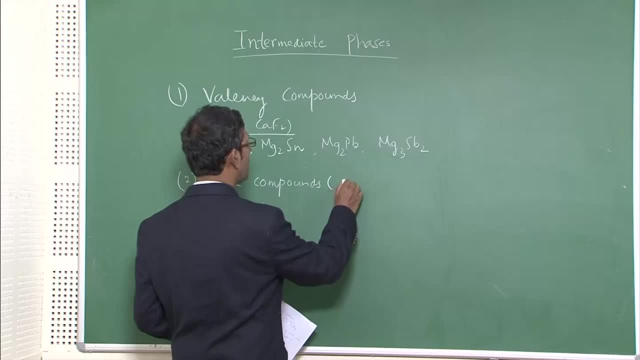 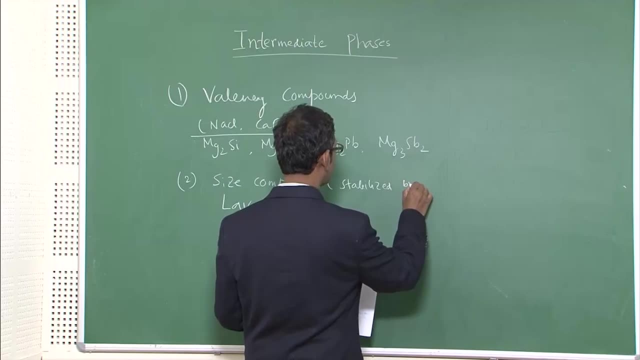 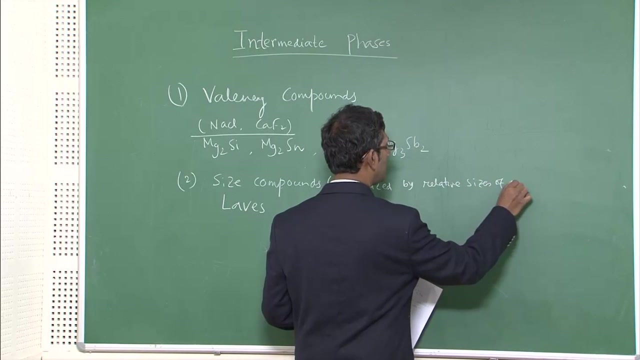 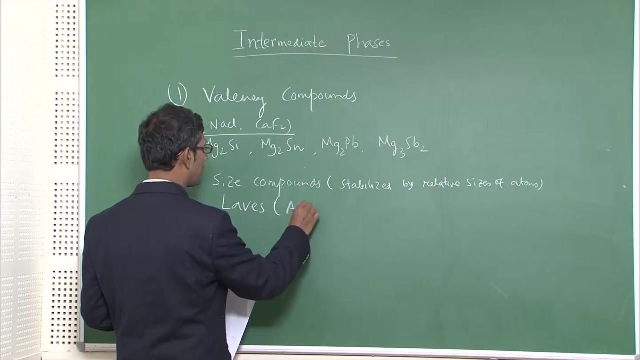 discovered these phases. that is why it is called lavish phases, So they are stabilized by size difference, relative sizes of the atoms, correct? there are two types of lavish phases and they, all of them, will have a composition: AB2 type. all of them- that is another classic, another important aspect of lavish phase- all of them will have. 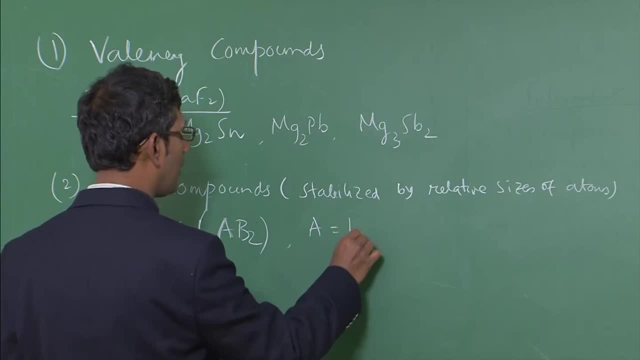 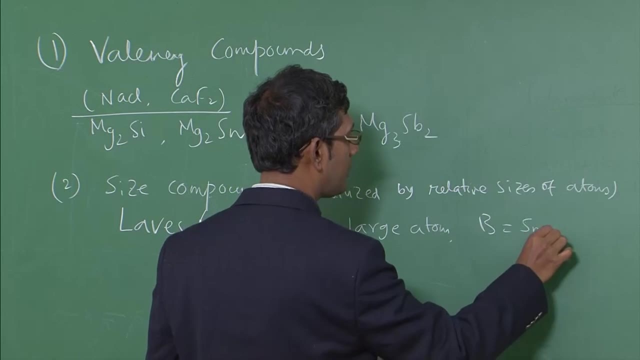 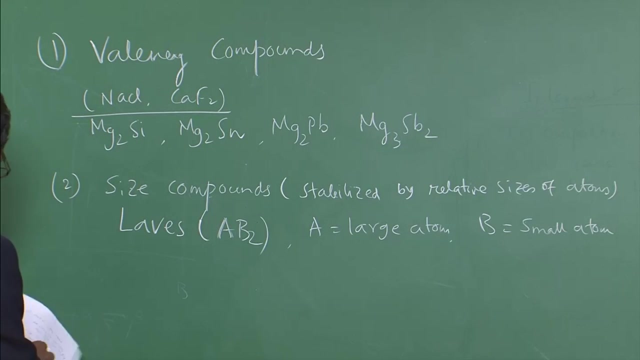 composition AB2 type, Where A is the Yes, Yes, Yes, Yes, Yes- Large atom and B is the small atom. okay, very simple to remember: AB2.. Now, what are these are? okay, these are very simple. there are many examples. first, let me. 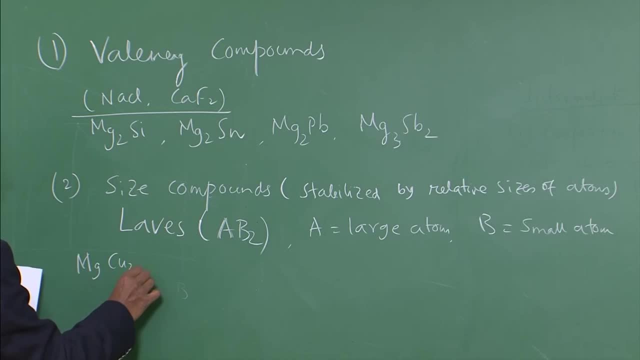 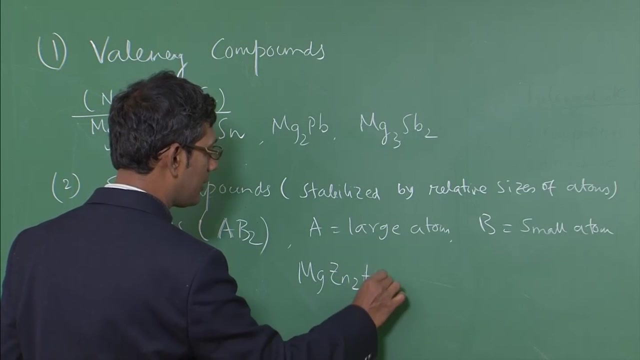 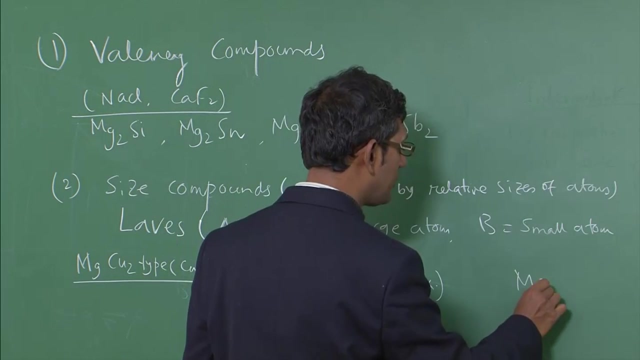 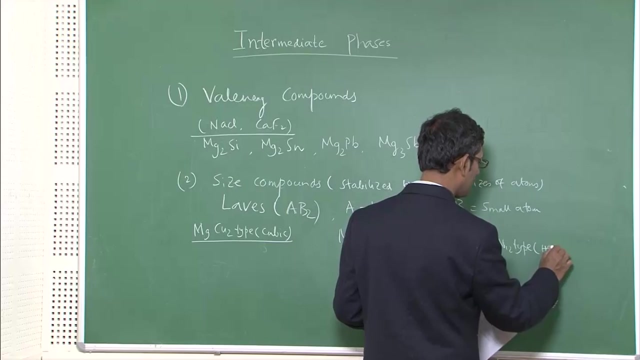 give the example. then I will talk about the structures: NGCU2 type. they are cubic. and then this is MgZn2 type. MgZn2 type. these are hexagonal. and last one is MgNi2 type. this is also hexagonal, but double unit cell, which we will show you later, or maybe today itself, is possible. this 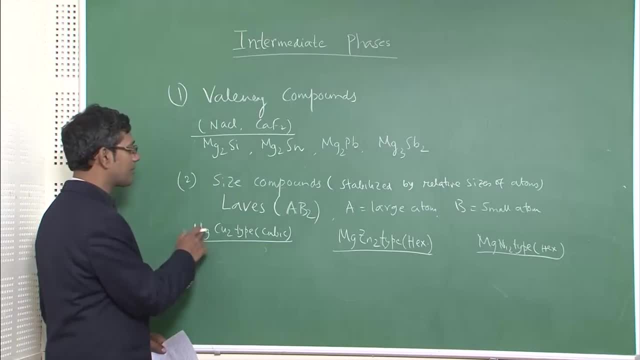 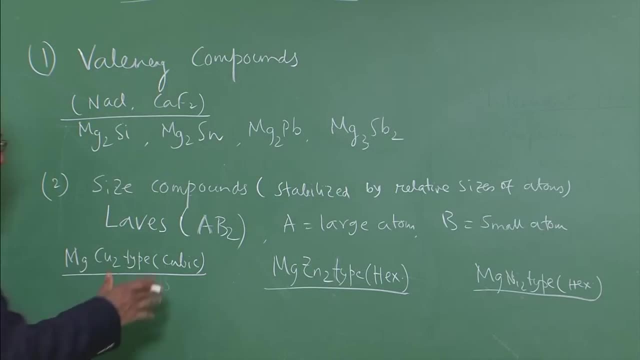 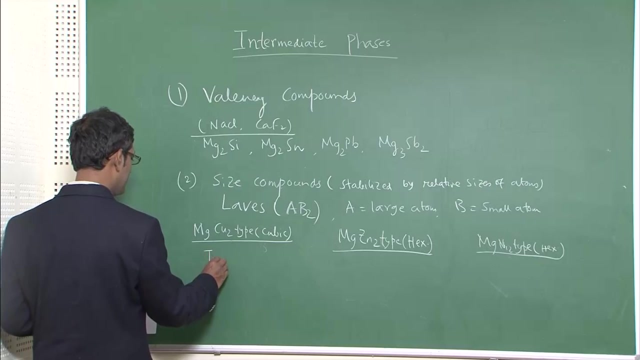 is lecture. So this is cubic. all of them has composition H2O, MgC2, MgZn2, MgNi2, all of them, So all of them can connect all the cubic phases which of this type size factor can be classified under MgC2. they are titanium, beryllium 2, silver beryllium 2 and bismuth, gold 2, all cubic and 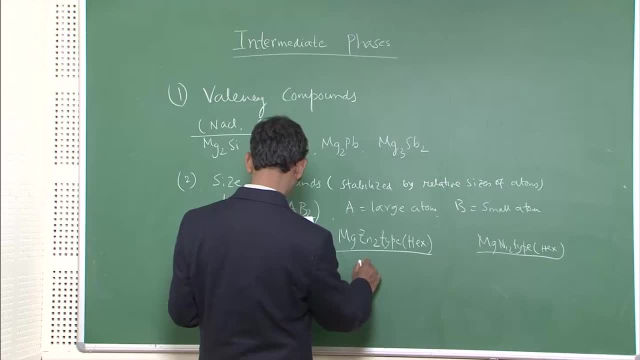 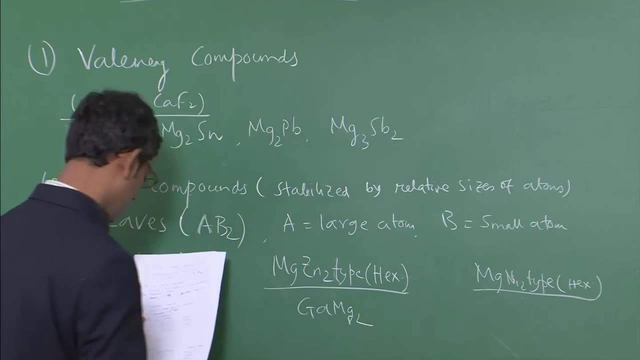 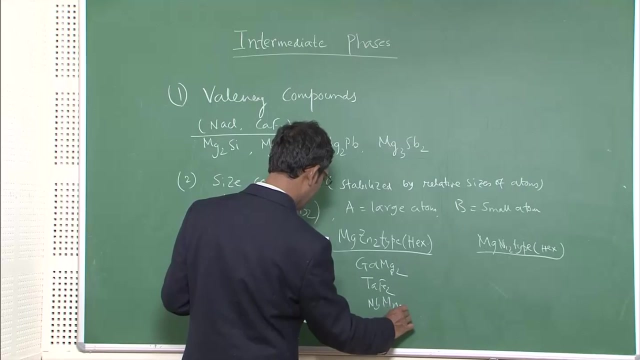 all of them have similar structure. Here this is silver beryllium 2 and bismuth gold 2, all cubic and all of them have similar structure. So this is gallium manganese- sorry, manganese M2, tantalum, Fe2 and niobium manganese 2, some 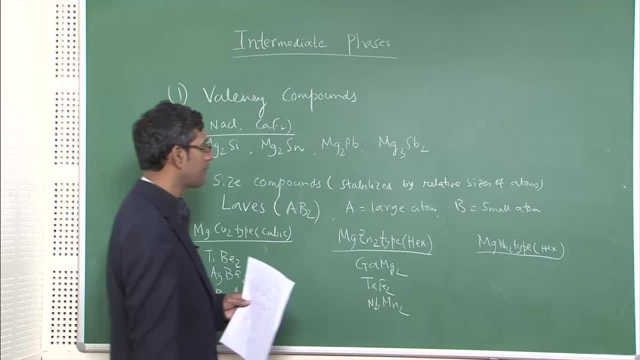 of them are superconductors, by the way, and some of them are very interesting materials. The last category is NdZn2, selenium, Rn2 and rn2.. So these are the two categories. So this is the two categories. So these are the two categories. 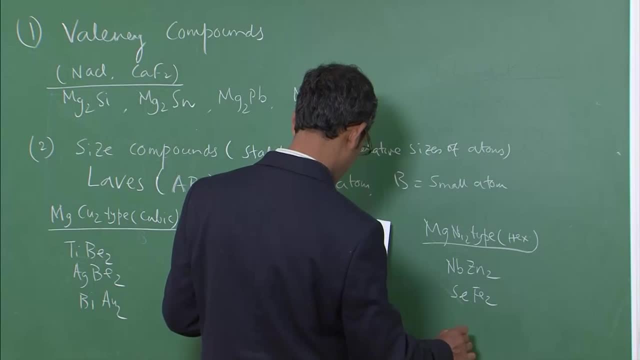 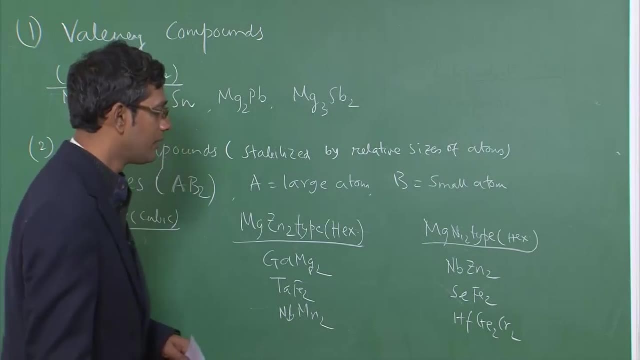 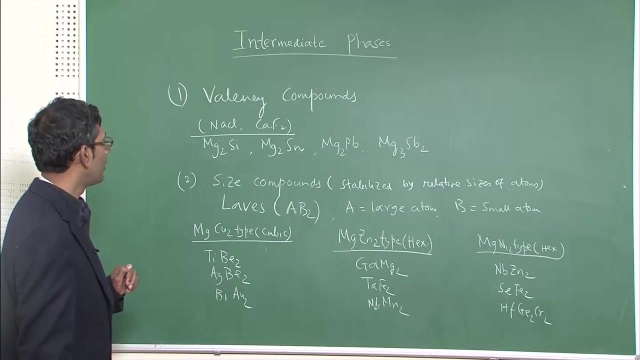 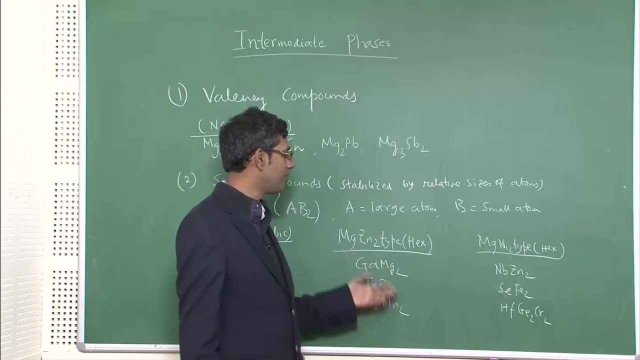 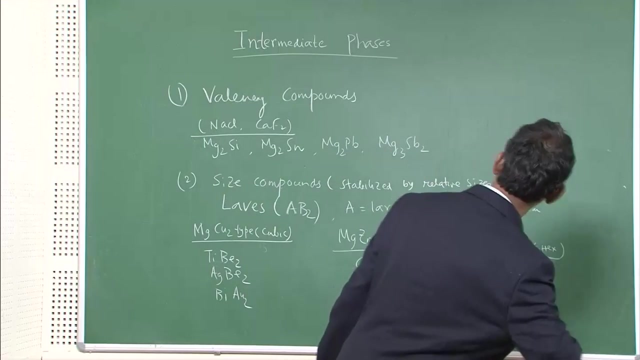 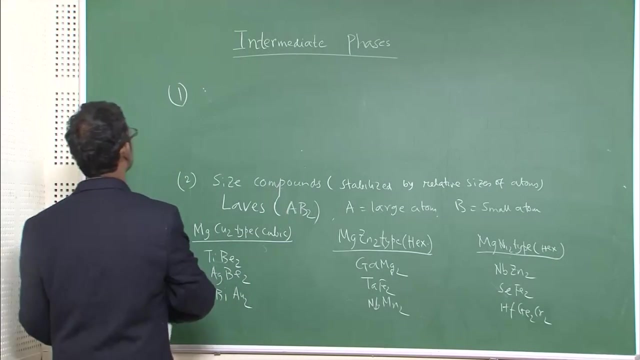 So this is the two categories, So this is the two categories, So this is the two categories. So there we have, and these are the examples. So last one is call valency a BCO3 component called electron compounds, because they are stabilized by electron to atom ratio. Electron compounds are. it is known as Hume-Rothery compounds- Hume-Rothery was the person who discovered it, Hume-Rothery compounds- and they are stabilized by E by A ratio. What is E by ratio? E is the valence electron, number of valence electron and A is the number. 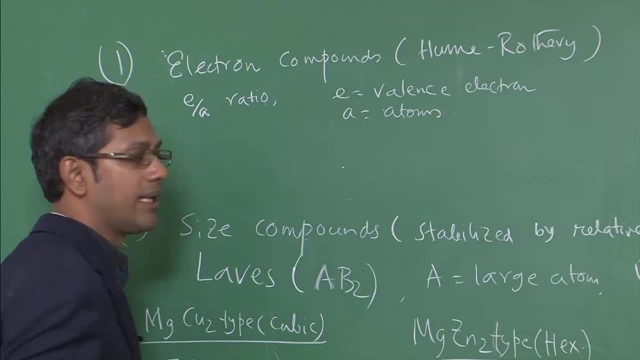 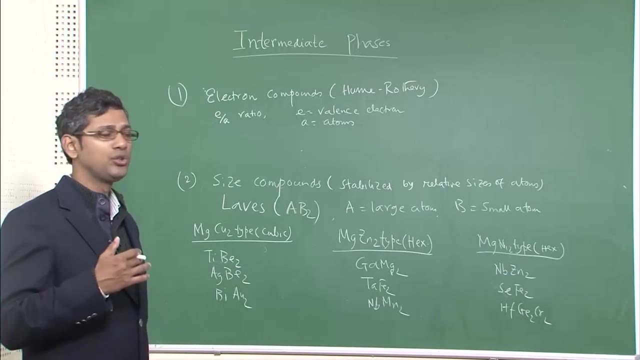 of atoms in the molecule. That is what is the factor which stabilizes. It is not easy to explain this. this basically depends on billion zone and the interaction between billion zone and the outer electron surface, The many things, But I am not going to detail of that. but this is mostly stabilized by E, by A ratio, and there. 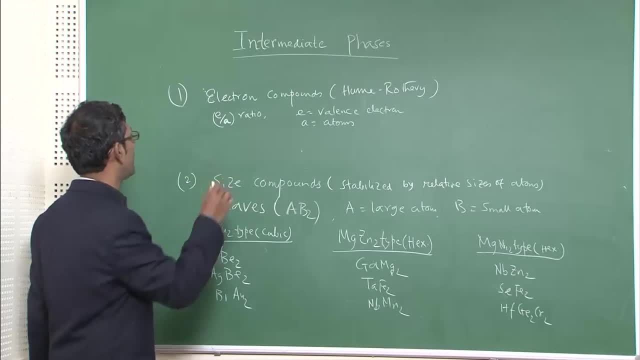 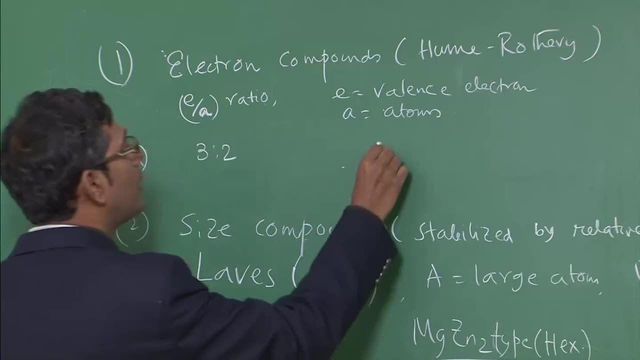 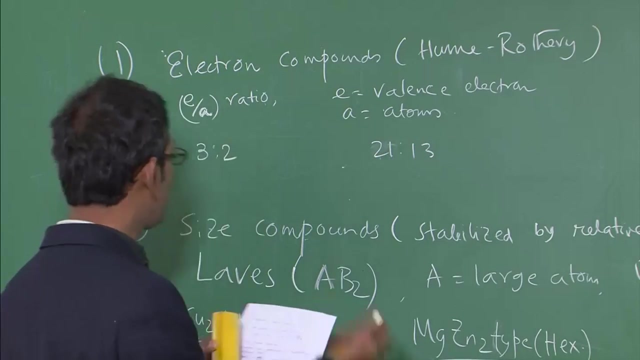 are 3 E by A ratio only at which this compound is stabilized. These 3 E by A ratios are: 3 is to 2, there are 3 E by A ratio: 3 is to 2,, 21 is to 13,, 21 is to 13 and last one is: 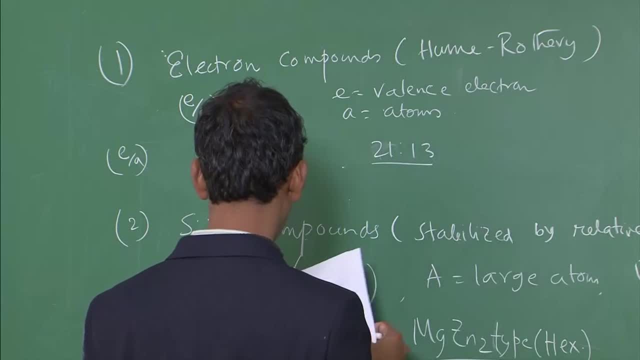 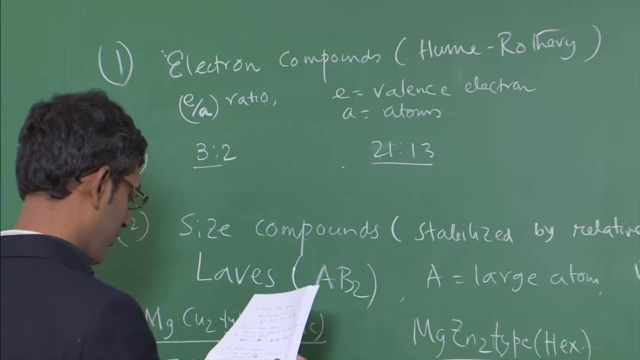 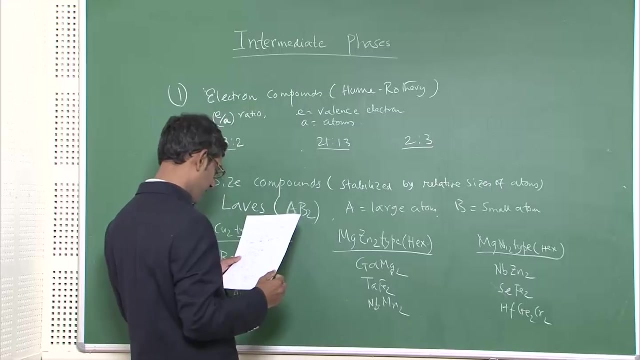 3 is to 2, 21 is to 13,. last one is something else. we will see. What is that. I think 2 by 3, yeah, correct. So there are 3 ratios, sorry, not 2 by 3, 7. 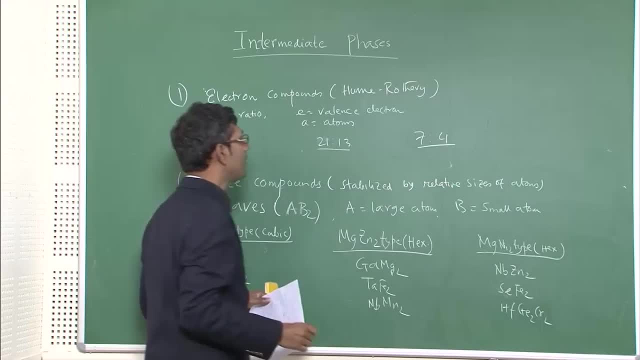 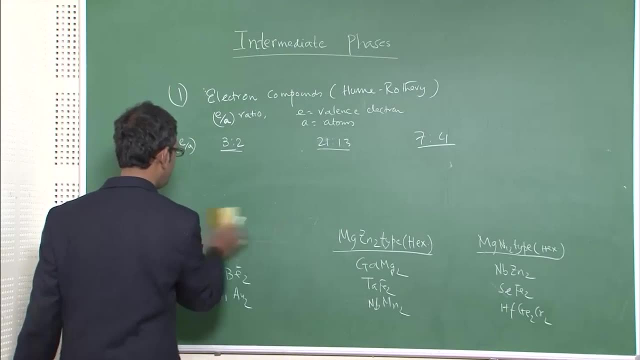 is to 4,- yeah, sometime I also forget- 7 is to 4, so there are 3 which this compounds are stable. So let us see some of the examples, which will be clear to you, correct? So first example of these: actually, 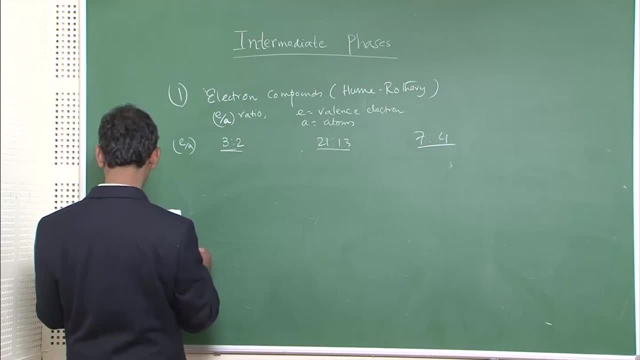 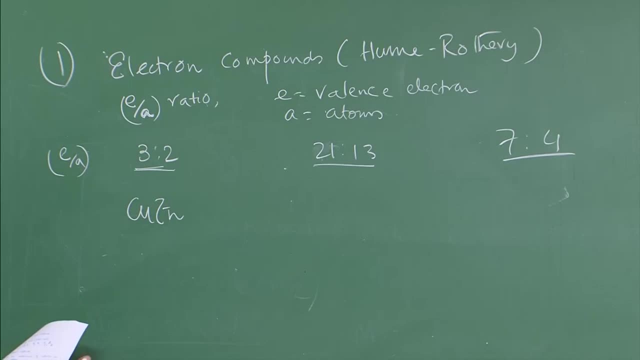 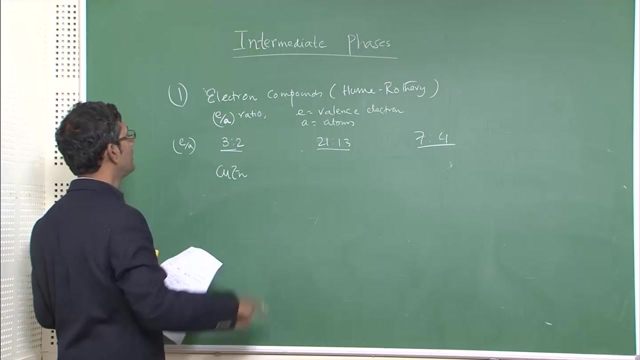 First example of this is. I will give you copper zinc. How it is 3 by 2?? There are 2 atoms. copper has 1 electron outer cell, zinc has 2 electron outer cell. so 2 plus 3 is 3 and 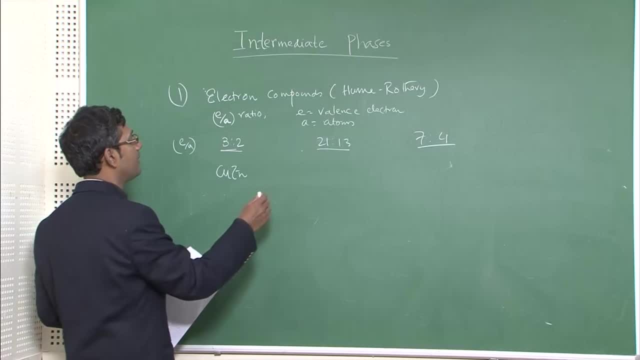 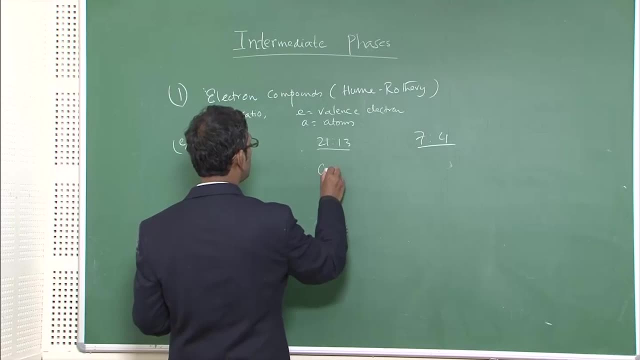 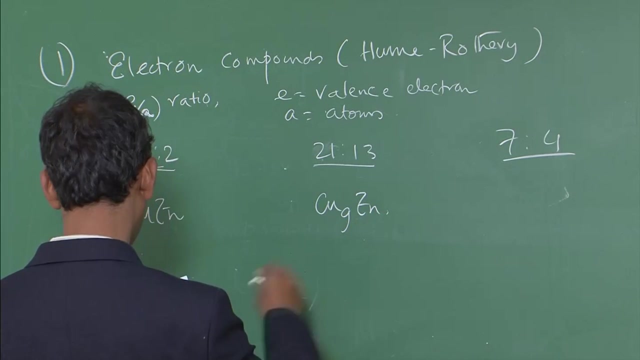 there are 2 atoms, so it is become 3 by 2.. So, and then this is another phase of copper zinc. Let me tell you Cu9Zn8,, Zn8, Zn. what is the number? Cu9, sorry, Cu9L4.. How it is. So, 9 plus 4 is 13. 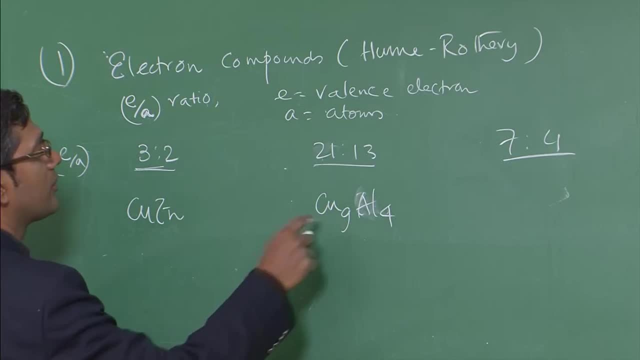 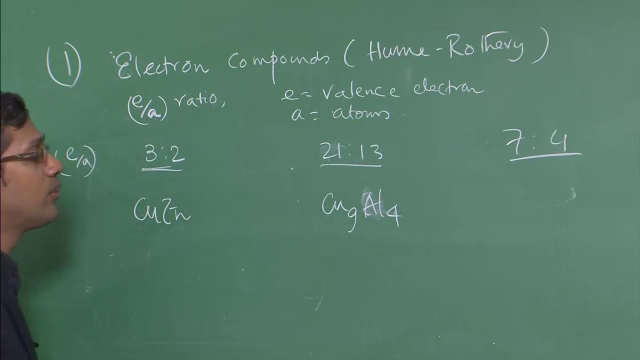 atoms in the unit A is 13 and 21 is how much 9, Cu has 1 electron, outer cell electron. so 9 into 1 and 4 into 3, 12. 12. 12 plus 9 is 21.. 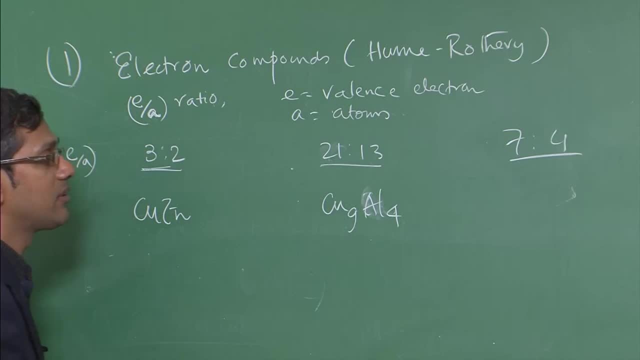 21.. 12 plus 9 is 1.. 12 plus 9 is 1.. 12 plus 9 is 1.. 12 plus 9 is 2.. 12 plus 9 is 2.. 12 plus 9 is 1.. 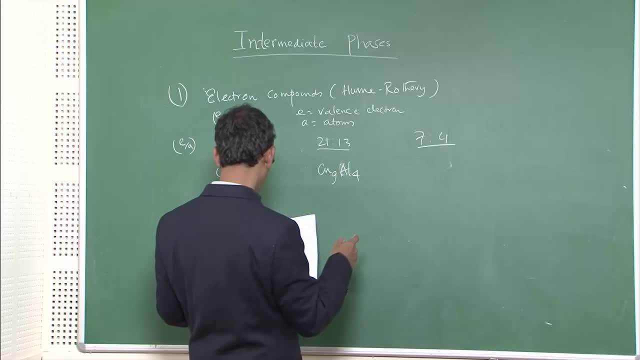 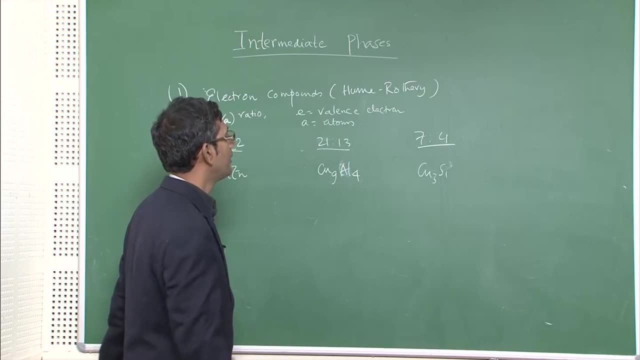 12 plus 9 is 2.. So it is 21 into 13.. That is what is stabilizing it. And let us see the 7 by 2,. okay, 7 by 2 is Cu3Si, How it is. 7 by 2 is 4.. 4 is always the 3 plus 1, is 4, 3 atoms of copper. 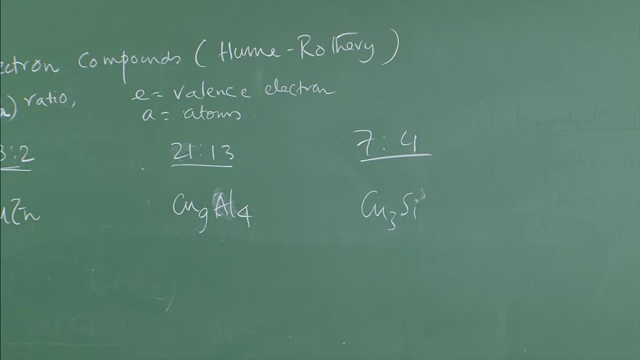 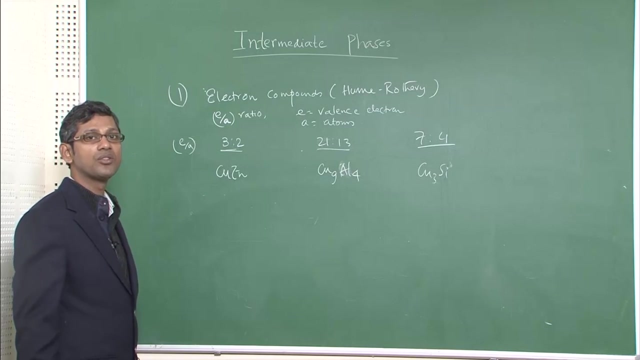 1 atom of silicon and the 7 is 3 plus silicon has 4 electrons outer cell. 7 plus 3 plus 4 is 7, so 7 electrons in outer cell divided by 4 atoms, correct? So this is what is the 3 ratios in which these compounds are stable and in the next class,